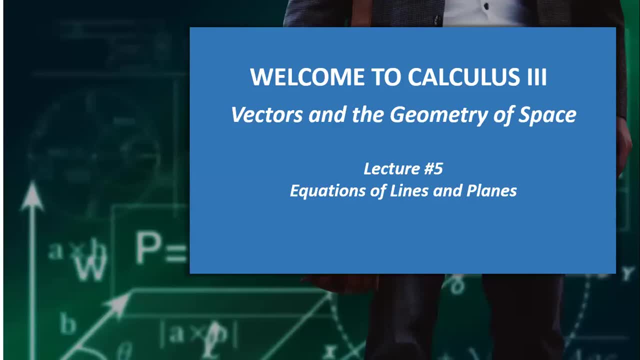 in the R3 space. Okay, so we're going to divide this lecture into two videos. So the first video we're going to talk about how to find the equations of the line in the R3, and then the second video we're going to work on how to find the planes. Okay, so now let's go to my 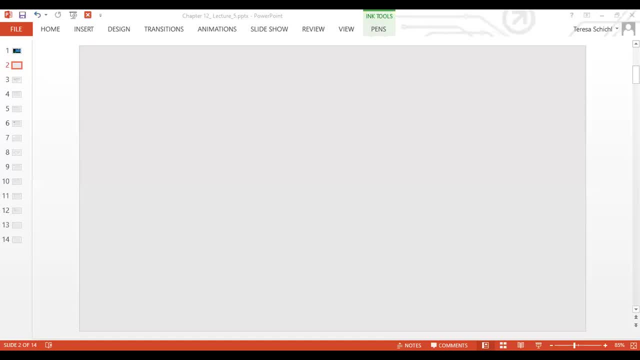 worksheets. So let's start. All right, so before we, you know, before we start to do the some problem, let's take a look, You know, in R3, right now we want to find the lines right, So let's kind of refresh back when we were. 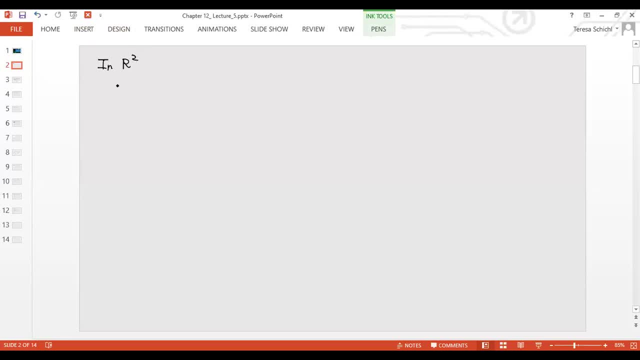 in high school we talked about the geometry in R2, so how do we find a line? So in R2, two, so, like in the geometry? we said: we always- you know the one of the formulas here- we say we can use the slope and one point right. so you give me one point. and so if this is x, one, y, one right. so 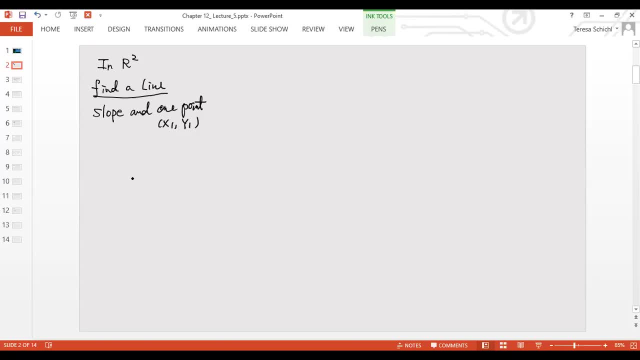 if you give me one point and you give me the slope, then i can know what is my lines looks like. right, so like in here. so that's why, if you have lines that go like here, right so for this line, see here. if you're passing through this specific point, x1, y1 and with the slope, let's say the slopes here is. 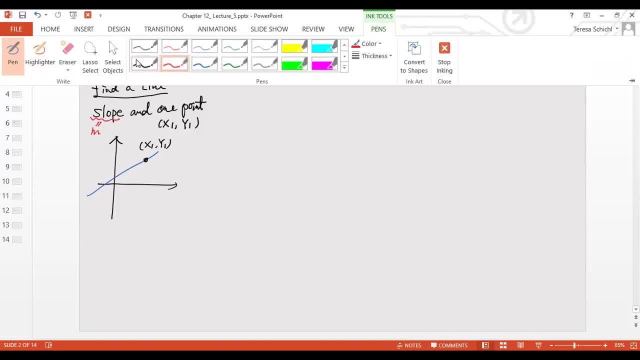 slope is: m see here. so now we all know the formulas here. we do so like that means for any points, right, so for any points in xy. so in order to represent this line, so what is the formula is we said: is y minus y1 equal to the? 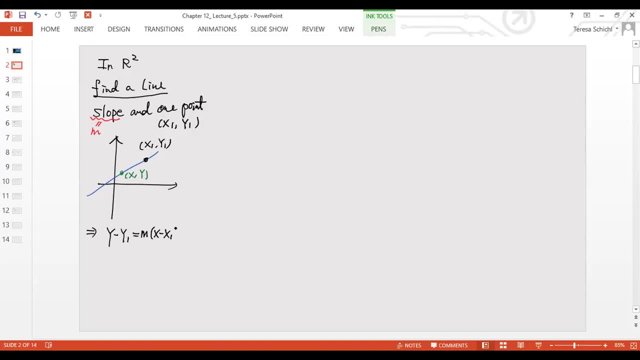 slope of x minus x ones here. right, this is what we call this: the slope and the intercept form. okay, now let's take a look in r3. right now, we expanding the r3s here. so how do i find it? i don't have to, so right now i have. 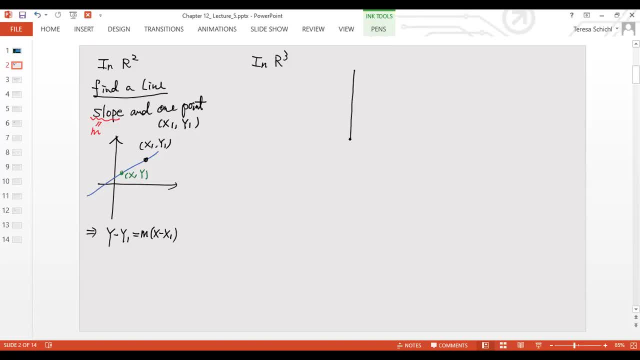 x, y and z's here, right? so let's take a look at these pictures here, okay? so here, this is my x, y and z. so this is my x, y and the z axis. so i have lines here. okay, so this line is in the space here, right? so now we have these lines here. 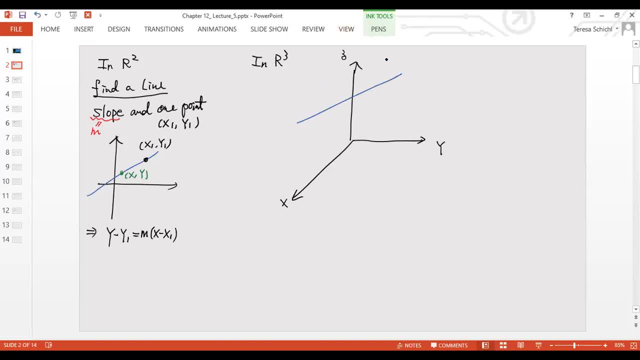 so i have this line okay, so these lines here, okay, so this is the line in the space. and then we say the same thing. you know the this line we know in order to define this lines right. so we say okay for this line. we know this line goes through a specific point. 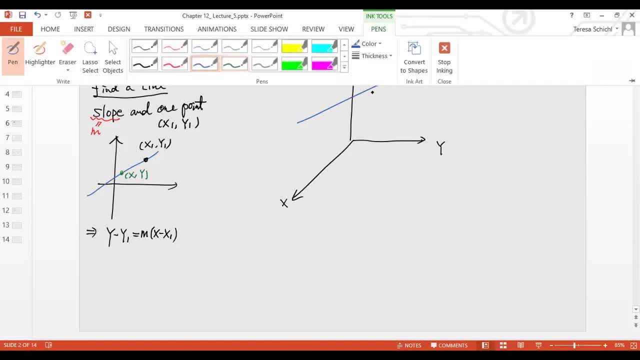 right. so the i say here: this line goes through these points here. okay, so this is the points. just like we talk about x1, y1s, here is the same. this is x0, y0, z0. right, so this is the point. this line goes through here. okay, and now in here and um, so the like: uh, let me write this point, uh. 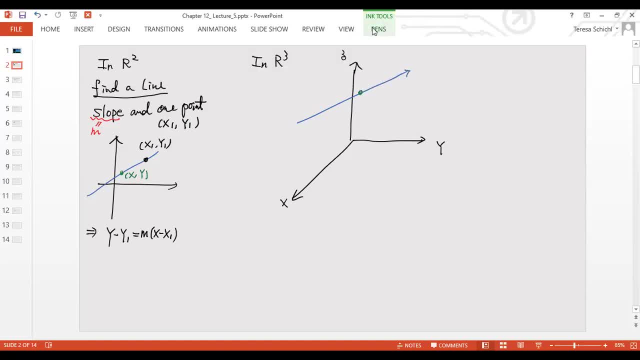 so, so it's not too crowded here, right, okay. so like this one's, here we say: this is the point, point x, zero, y zero and the z: zero. so here, okay, and now in here. now in here we say okay, so this line going to passing this point here and also right, you know, like in r2, you need to know which. 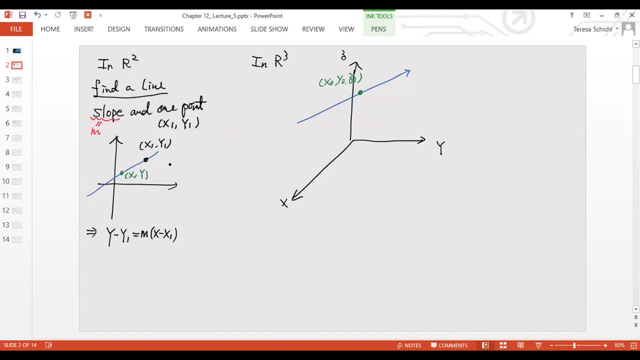 direction, this line goes right. so the this: you know, like that's why in r2 we have a slope. so for you here we say, okay, this line go, this directions right, okay. so i want to uh, make a kind of. so we will define this as a cross-sectional line. 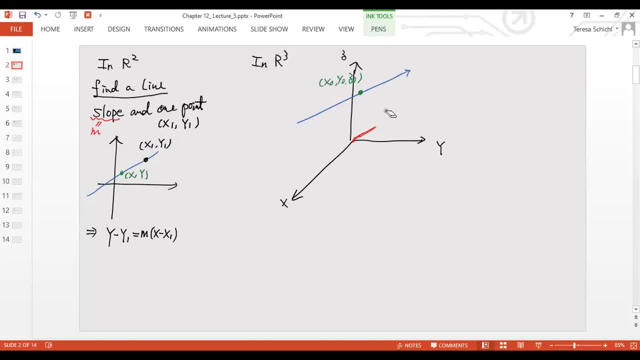 so i'm going to have vectors here. this vector i said this is what i call the v vectors here. okay, so this is the v vector. and the v vector is made of the a, b, c points, right? so this is a vector abc, here z equal to c. so this one parallel to the given lines here. so this is what i call this, the v. 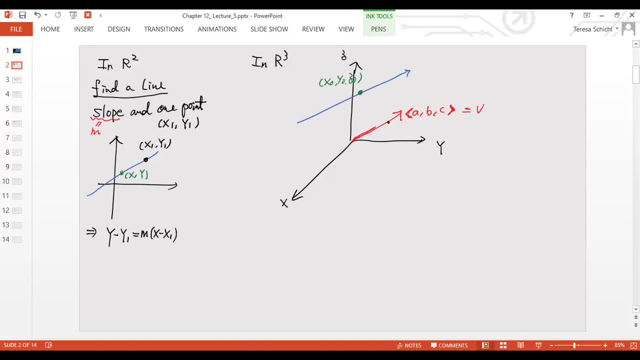 vector because this line going to parallel to this v vectors here, correct. so this v vectors here, that's what we call the busy is the direction. so this is we call this is a direction vector. so it's the very similar concept, like the slope, but this is the direction vectors here. so, like the name here is a, b, c, like those are the directions. 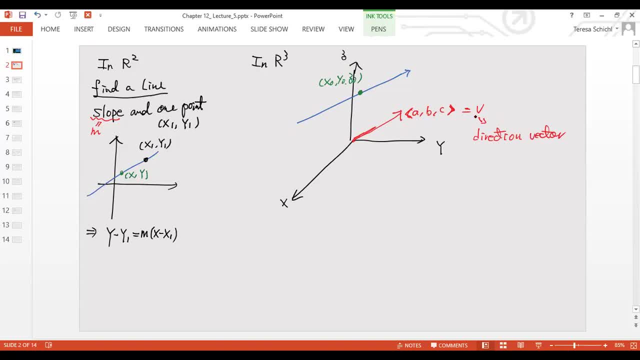 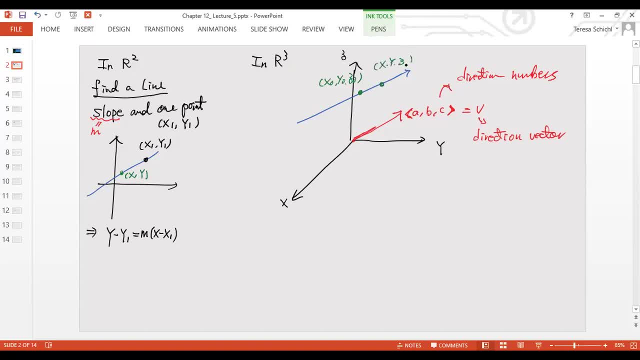 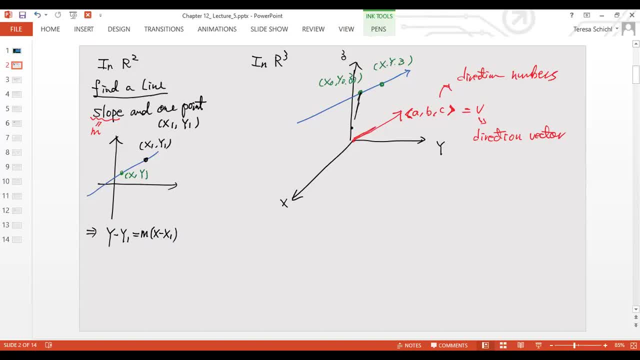 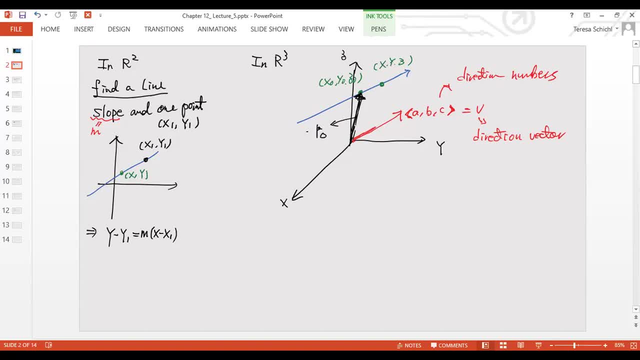 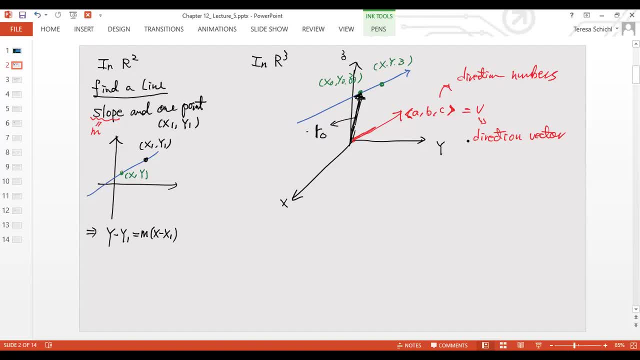 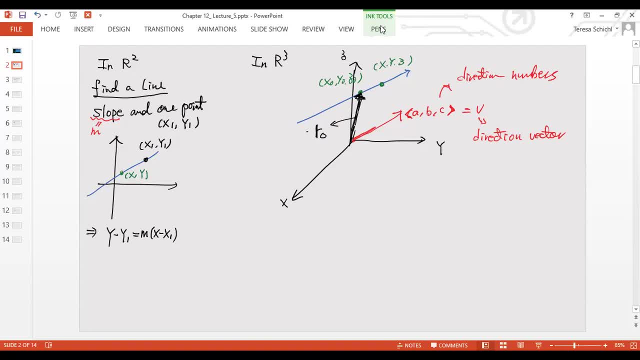 so this is the direction vector vectors here and now. okay, so this is the v vector. so this is the direction vector vectors here and now. okay, so this is the v vector. so i know because the v is so, i know because the v is so, i know because the v is parallel to here. so i know for. 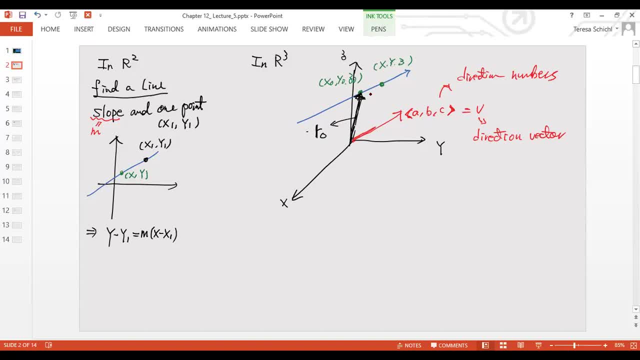 parallel to here, so i know for parallel to here. so i know for every you know any points here, right. so every you know any points here, right. so every you know any points here, right. so you can always, you can always, you can always, right, so you can always. let me see how do i. 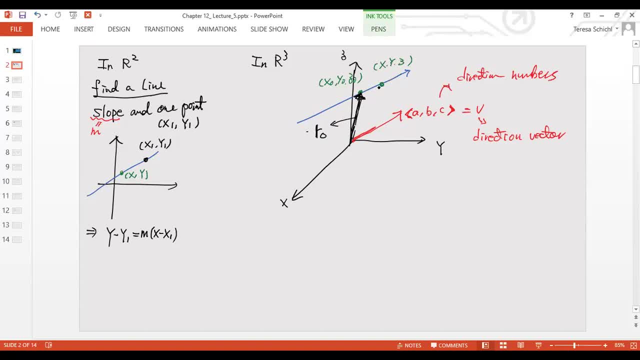 right. so you can always let me see how do i right. so you can always let me see how do i do this, do this, do this by the color. okay. so for any point x, y by the color. okay. so for any point x, y by the color. okay, so for any point x, y, z, here you can always. 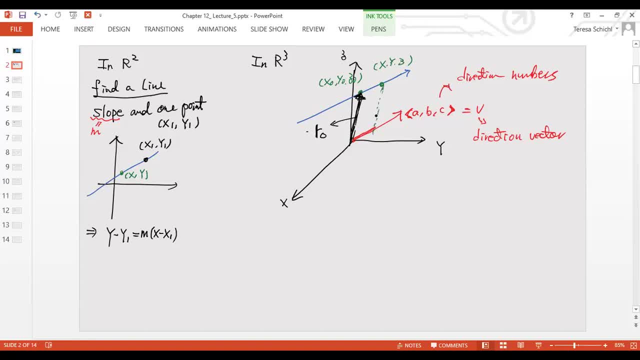 z here you can always z here you can always parallelogram like here, parallelogram like here, parallelogram like here, right. so they will be what this diagonal right, so they will be what this diagonal right, so they will be what this diagonal, that's will be there. so this is: how do i? 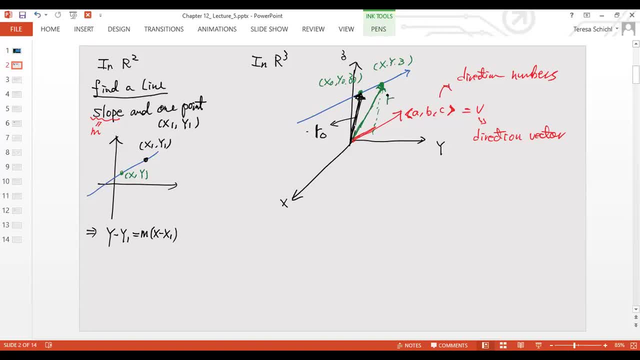 that's will be there, so this is how do i. that's will be there, so this is how do i define the lines right. so this is i call: define the lines right. so this is i call: define the lines right. so this is i call. this is the rr. 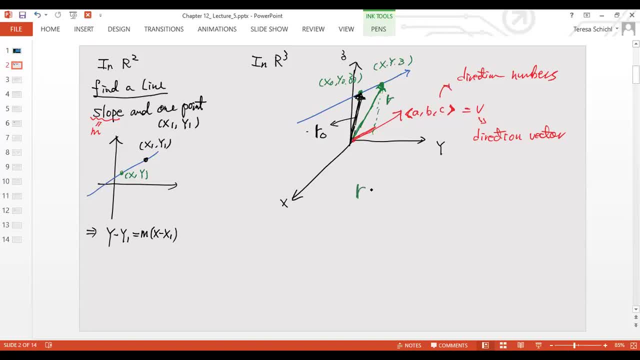 this is the rr. this is the rr, right. so i know the rr, right. so i know the rr right. so i know the rr is always equal to the diagonal. it's is always equal to the diagonal. it's is always equal to the diagonal. it's always equal to sides here, right? so it's. 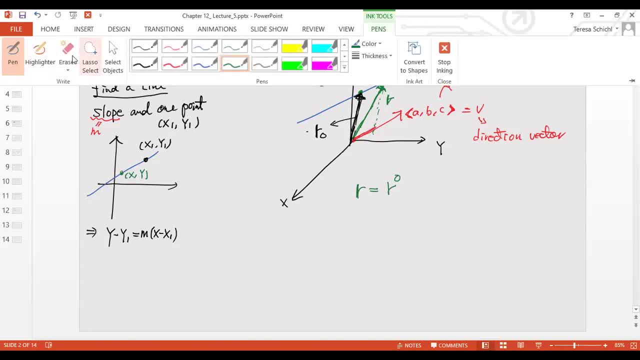 always equal to sides here, right? so it's always equal to sides here, right? so it's a r zero. okay, so it's a a r zero. okay, so it's a r zero. okay, so it's a r zero. a r zero. okay, so it's a r zero. okay, so let me put the zero i should put. 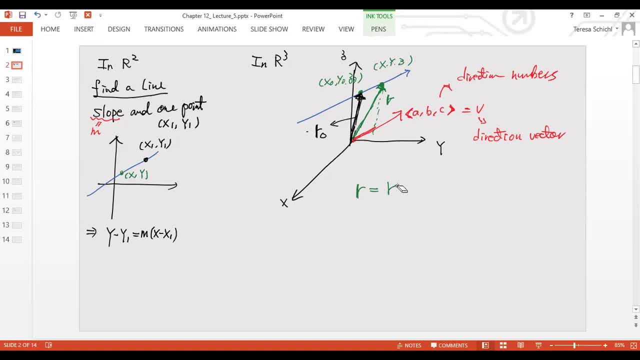 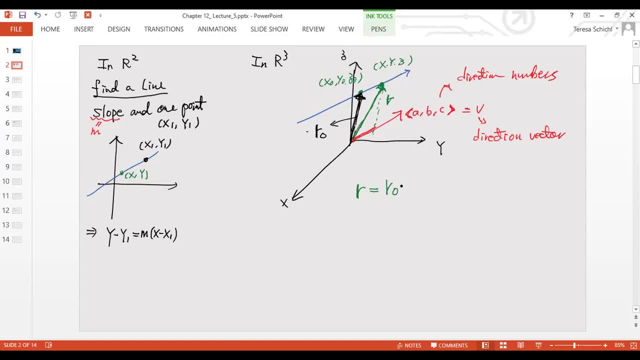 in the bottom here, right. so so it's r zero and the plus so it's r zero and the plus, so it's r zero and the plus right, plus right, plus right, plus. so plus these factors here, plus this, so plus these factors here, plus this, so plus these factors here, plus this vector. 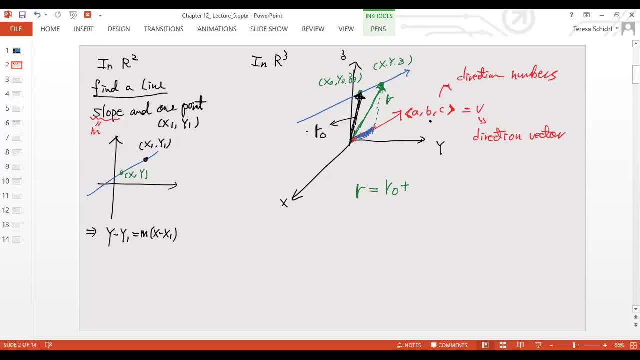 vector vector. so this vector is a part of, so this vector is a part of, so this vector is a part of the directional vectors. right so, but the directional vectors, right so, but the directional vectors, right so, but the xyz can be anywhere, so the xyz can be anywhere, so. 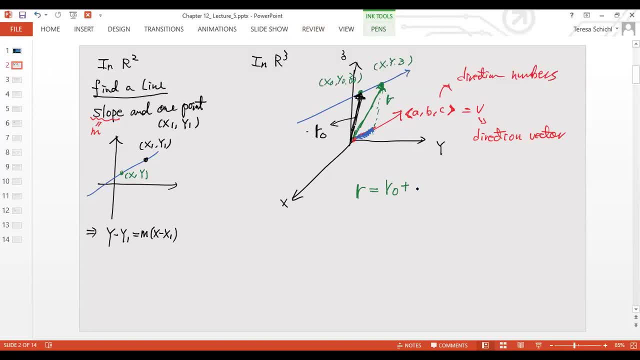 the xyz can be anywhere. so that's why what i'm, that's why what i'm, that's why what i'm plus in here, i plus the t plus in here, i plus the t plus in here, i plus the t times. what t times these times. what t times these. 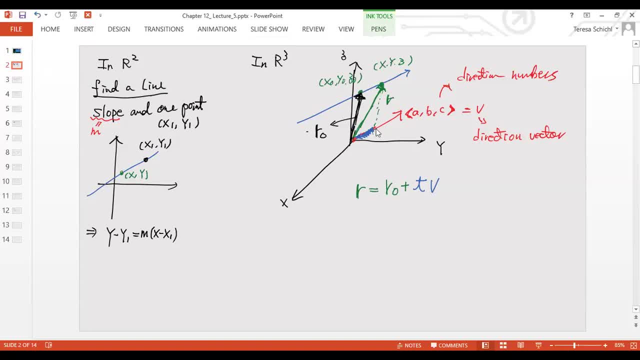 times what t times these here right, so like in here. so t here right, so like in here, so t here right, so like in here. so t could be one half because this is the could be one half, because this is the could be one half because this is the v's right. so that's why. 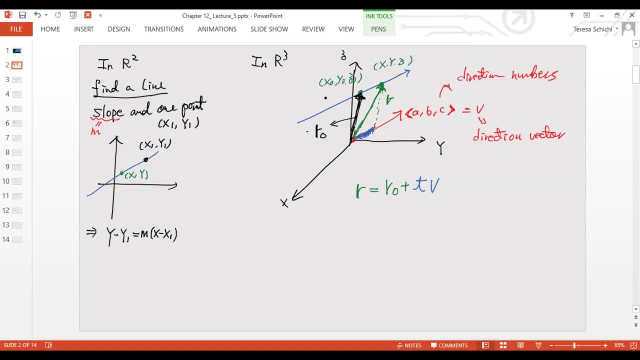 v's right. so that's why v's right. so that's why this is what i call. it is the. this is what i call. it is the. this is what i call. it is the vector's form about the line all right. vector's form about the line, all right. 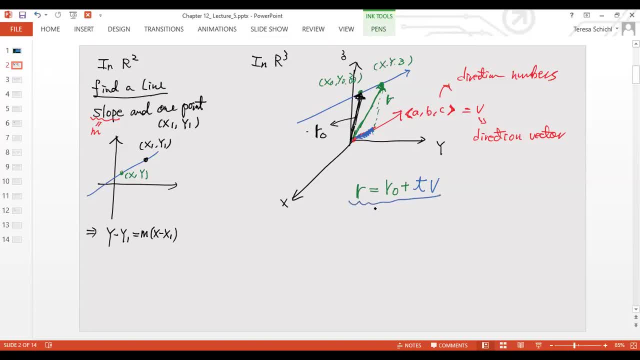 vector's form about the line: all right, so let's take a look. so this is the. so let's take a look. so this is the. so let's take a look. so this is the vector's form. vector's form, vector's form. okay, so this is a vector's form. how do 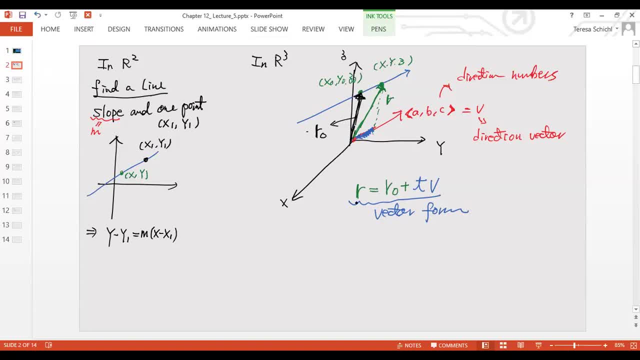 okay, so this is a vector's form. how do? okay, so this is a vector's form. how do we define the line? we define the line, we define the line. so what is r0 here? r0 is the vector. so what is r0 here? r0 is the vector. 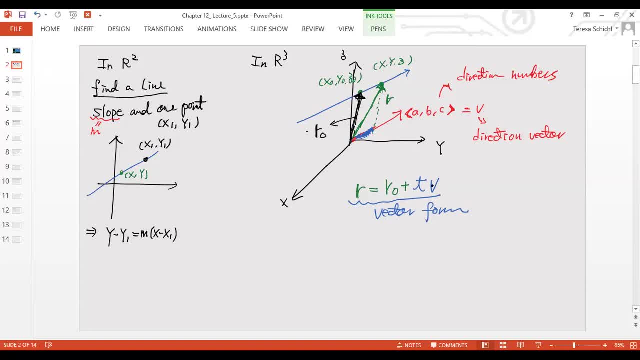 so what is r0 here? r0 is the vector, the point. you know this line going to the point, you know this line going to the point, you know this line going to go through. what is the v go through? what is the v go through? what is the v? v is the directional vector. so it's. 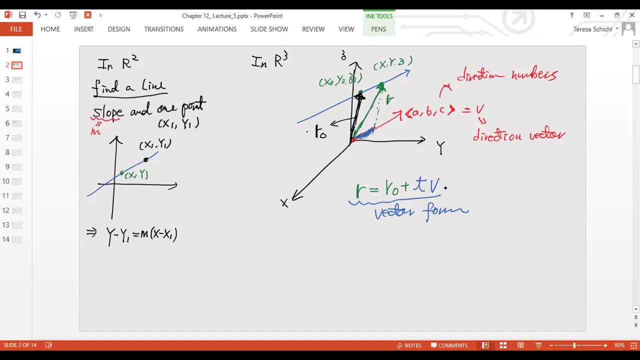 v is the directional vector, so it's v is the directional vector, so it's very similar, like very similar, like very similar, like here- right, it's a point and a slope here, right, it's a point and a slope here, right, it's a point and a slope, right. but 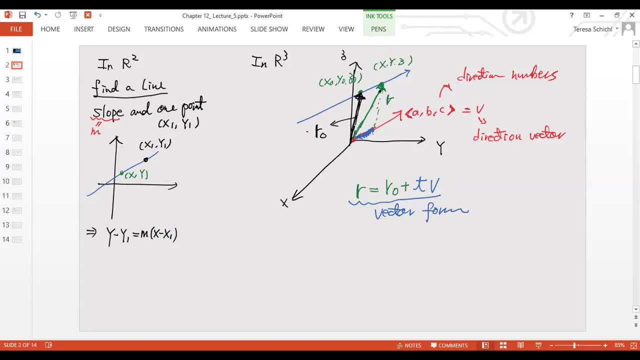 right, but right. but here we call this directions here. so here we call this directions here. so here we call this directions here. so now, if you kind of now, if you kind of now, if you kind of write it out, then here you will see write it out, then here you will see. 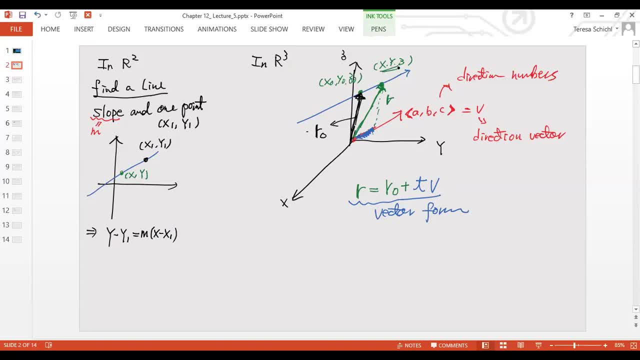 write it out, then here you will see here. so what is the r here? so what is the r here. so what is the r? i is any point x, y, z is right. so you, i is any point x, y, z is right. so you, i is any point x, y, z is right. so you will say: this is x, y. 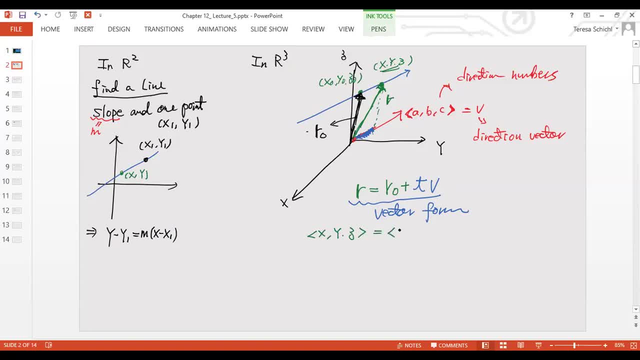 will say this is x. y will say this is x? y. z is equal to what is the r zero. is z is equal to what is the r zero. is z is equal to what is the r zero is the point you go through, so it's y. 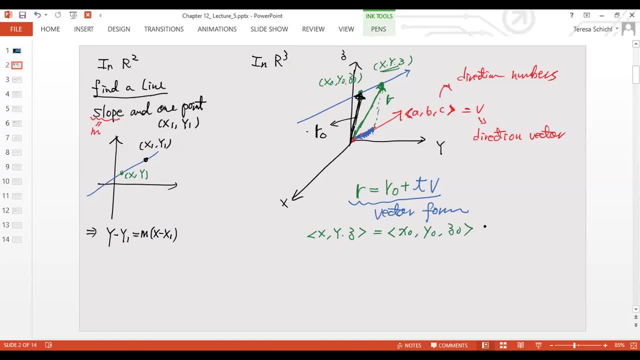 the point you go through, so it's y. the point you go through, so it's y. zero z zeros right and the plus zero z zeros right and the plus zero z zeros right and the plus the t, that's the parametric parameter. the t, that's the parametric parameter. 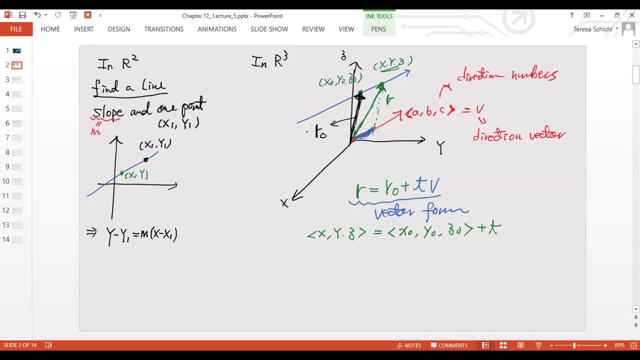 the t, that's the parametric parameter, so it's so, it's so, it's. he can be any numbers, right, okay, so the he can be any numbers, right okay. so the he can be any numbers, right okay. so the now in here, now in here, now in here in here, now let's see here this will. 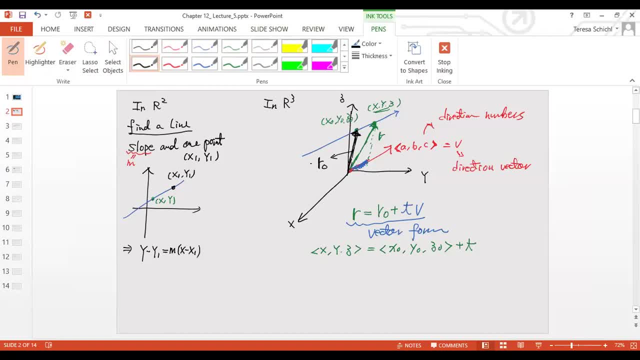 now, let's see here, this will now, let's see here, this will be: be: be okay so the okay. so this will be this okay, so the okay. so this will be this okay so the okay. so this will be this color, color, color. no, this color. all right, so this one's. 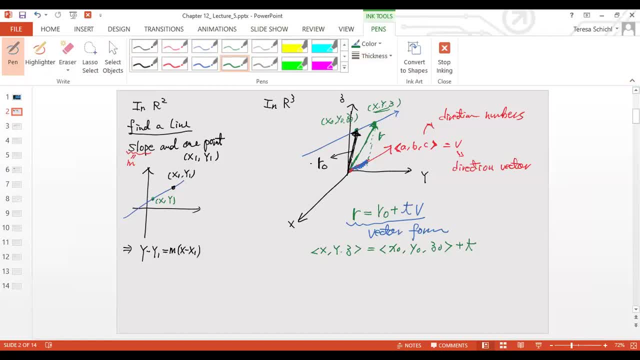 no, this color, all right, so this one's. no, this color, all right. so this one's here. the t, here, the t. here, the t will be, so the so t will be any number will be, so the so t will be any number will be, so the so t will be any number and the v. 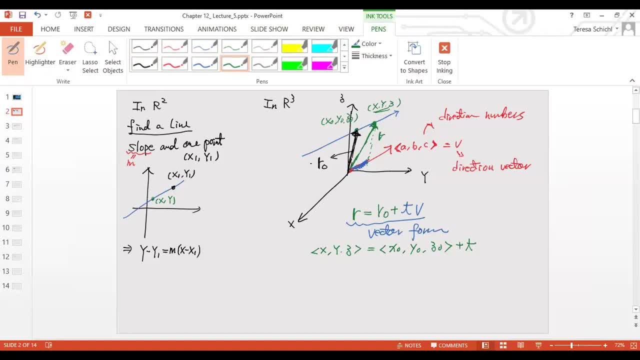 and the v, and the v will be our directional vectors, will be our directional vectors, will be our directional vectors. okay, so the v is our directional. okay, so the v is our directional. okay, so the v is our directional vectors. right, so that's why. vectors, right, so that's why. 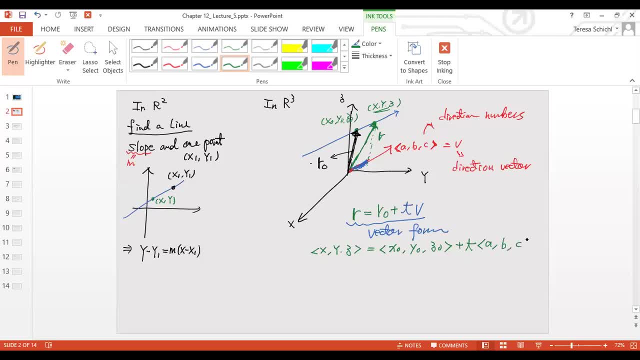 vectors, right. so that's why it will be a b, it will be a b, it will be a b. c here: correct now. you can put it like c here, correct now. you can put it like c here, correct now. you can put it like this way, this way. 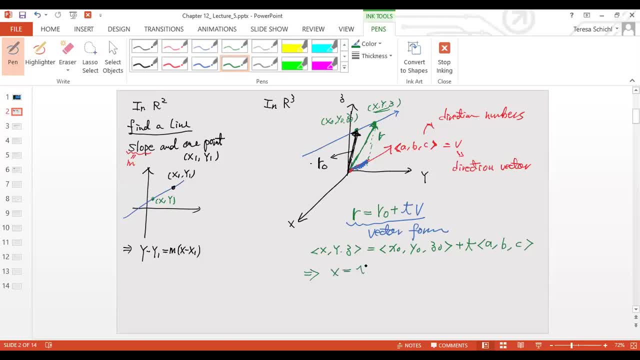 this way: here we'll say x is equal to. here we'll say x is equal to. here we'll say x is equal to x0 plus t a, x0 plus t a, x0 plus t, a and y is equal to and y is equal to. 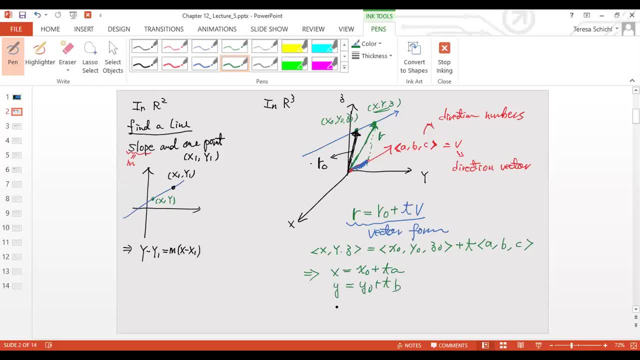 and y is equal to y0 plus tb, y0 plus tb, y0 plus tb. z is equal to z0 plus z is equal to z0 plus z is equal to z0 plus tc. and, like i said the t here right tc. and like i said the t here right. 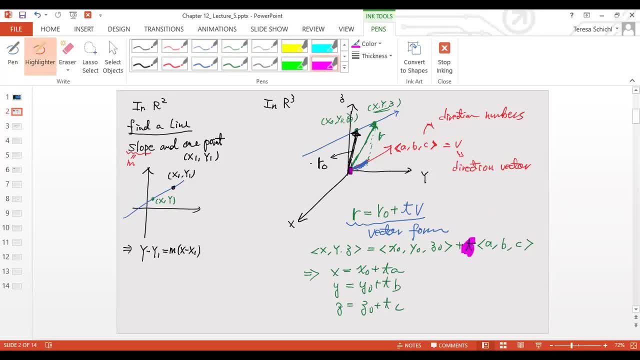 tc and, like i said, the t here right so the. so the t here right so the. so the t here right. so the t here. this is the t here, this is the t here, this is the parameter. so this is what we call the parameter, so this is what we call the. 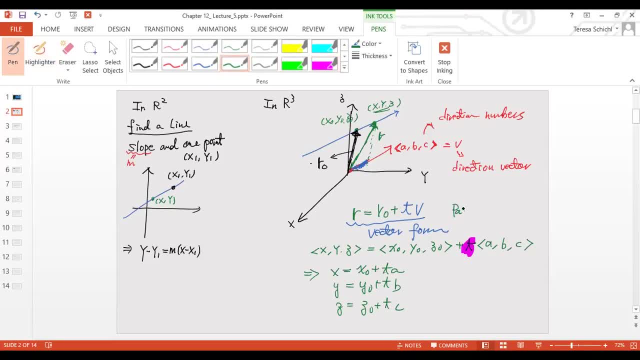 parameter. so this is what we call the. what this is, we call is a parametric. what this is we call is a parametric. what this is we call is a parametric form. okay, so this is a parametric form. okay, so this is a parametric form. 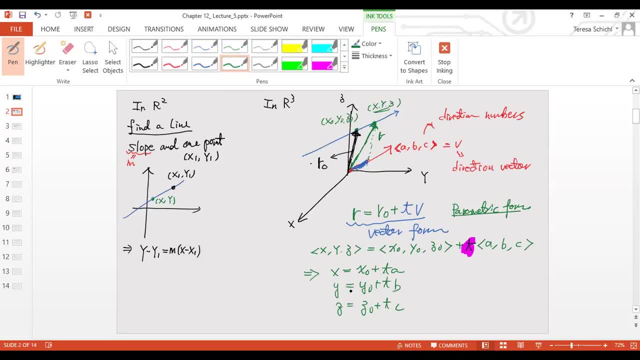 okay, so this is a parametric form. how do we write a x? how do we write a x? how do we write a x? you know how do we write a lines, right? you know how do we write a lines, right? you know how do we write a lines, right? so the line is x, y, z. 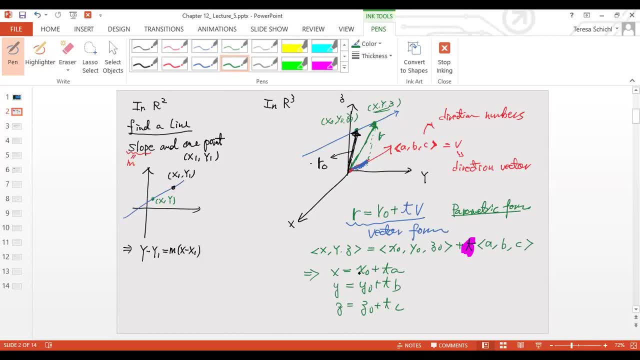 so the line is x y z, so the line is x y z, so this is a very similar. like like the, so this is a very similar, like like the, so this is a very similar. like like the slope intercept form right, so similar. slope intercept form right, so similar. 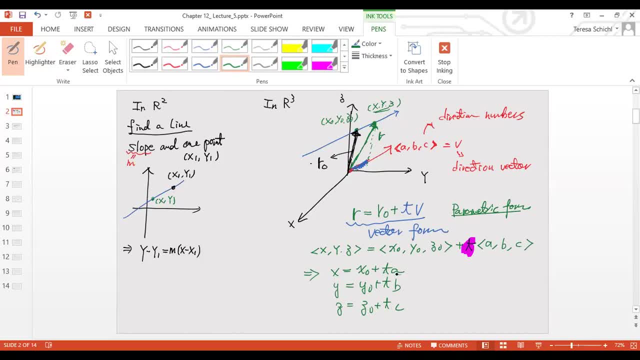 slope intercept form right. so similar like that. like that, like that x equal to x 0 plus t a, because the a x equal to x 0 plus t a, because the a x equal to x 0 plus t a, because the a here is what is the directional. so it's. 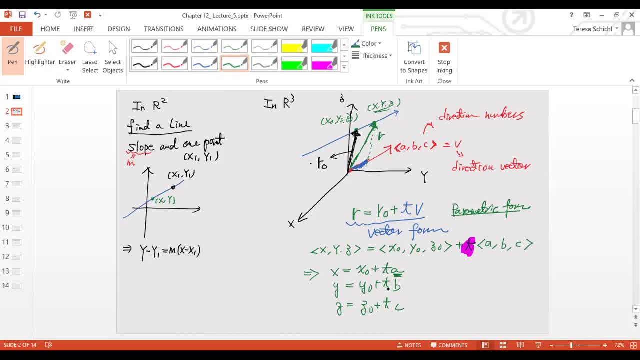 here is what is the directional. so it's. here is what is the directional. so it's kind of the slope right, kind of the slope right, kind of the slope right. now y is the y 0 plus t b's right. so now y is the y 0 plus t b's right. so 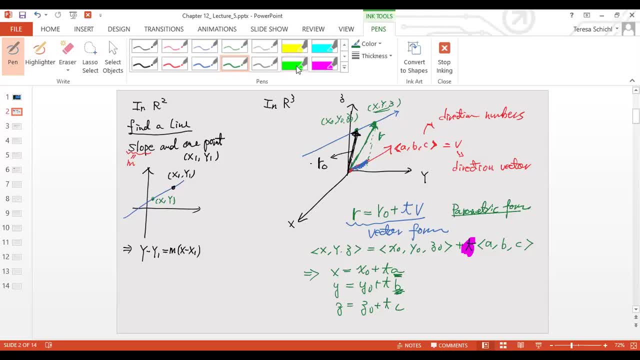 now y is the y 0 plus t b's right, so it's kind of like the slope for the b. it's kind of like the slope for the b. it's kind of like the slope for the b, i mean the kind of like it's not risk. i mean the kind of like it's not risk. i mean the kind of like it's not risk, you know, so we don't want to use the. you know so we don't want to use the. you know so we don't want to use the word of the slope. 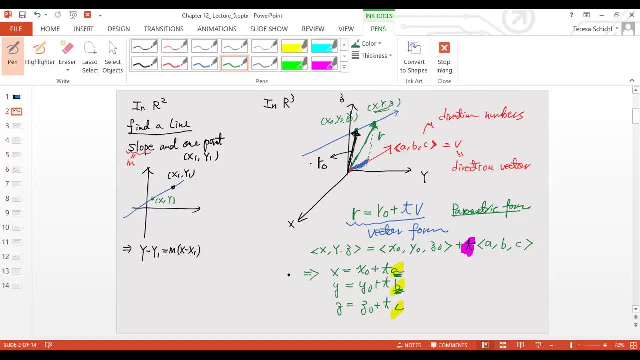 word of the slope, word of the slope, but this is what we're coding. is the but this is what we're coding. is the but this is what we're coding. is the directional vector, directional vector, directional vector: right directional parameters here. so right directional parameters here. so. 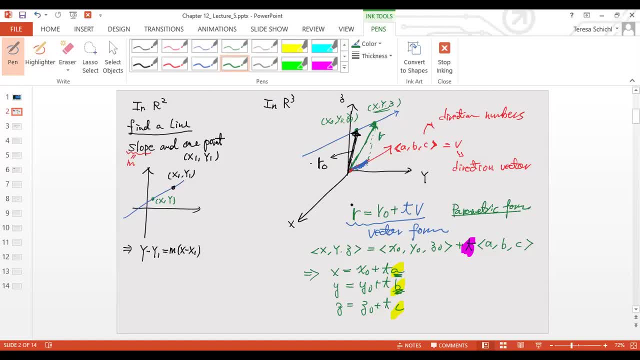 right directional parameters here. so this is the parametric, this is the parametric, this is the parametric. forms here, so we have two forms right, so forms. here, so we have two forms right so forms. here, so we have two forms right, so the here, this is the vector forms. 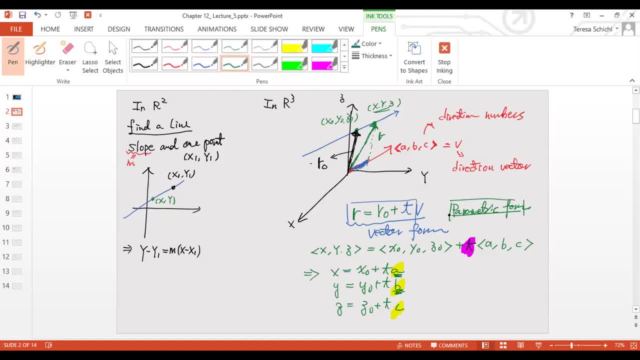 the here, this is the vector forms. the here, this is the vector forms. so this one's your t. you can say the t, so this one's your t. you can say the t, so this one's your t. you can say the t is equal to what? 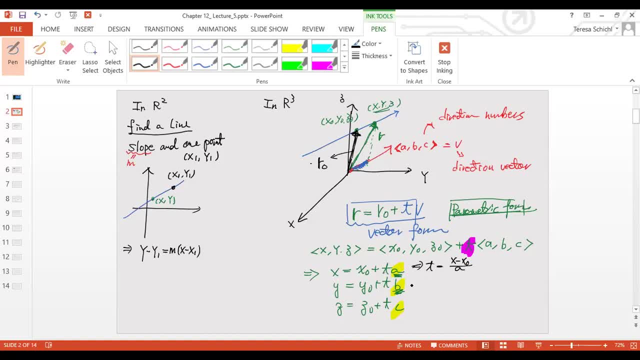 is equal to what is equal to what. x minus x zero divided by a. x minus x zero divided by a. x minus x zero divided by a. and this one's here t is equal to what. and this one's here t is equal to what. and this one's here t is equal to what. y minus y zero divided by b. 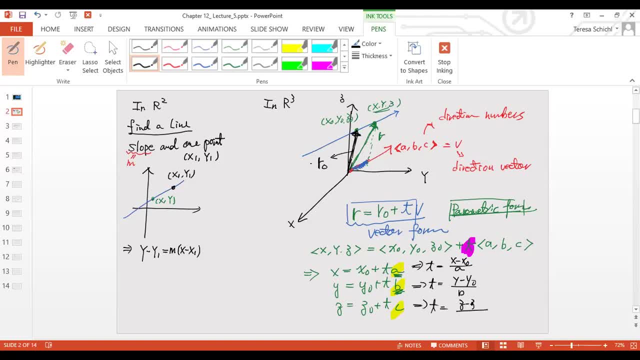 y minus y zero divided by b. y minus y zero divided by b. and the t is equal to what? and the t is equal to what? and the t is equal to what. z minus z zero divided by what divided. z minus z zero divided by what divided. 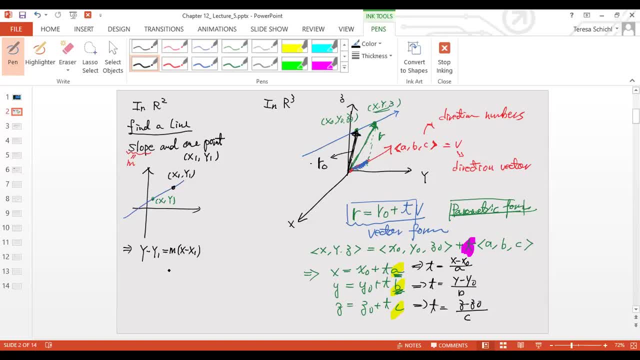 z minus z zero. divided by what? divided by c, by c, by c. as you can see, they are all equal to t. as you can see, they are all equal to t. as you can see, they are all equal to t. so that's why i can write it in here is: 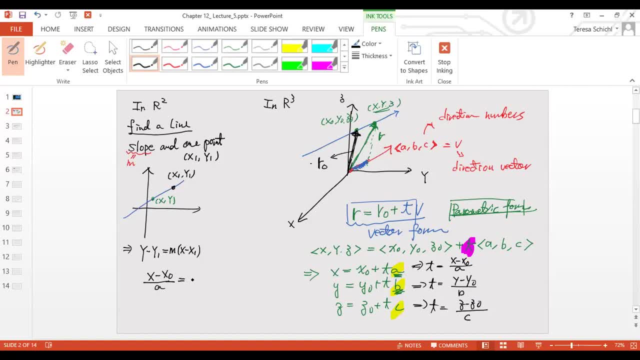 so that's why i can write it in here: is so that's why i can write it in here: is x x minus x, x, x minus x, x, x minus x. zero over a is equal. zero over a is equal. zero over a is equal y minus y. zero to the b. 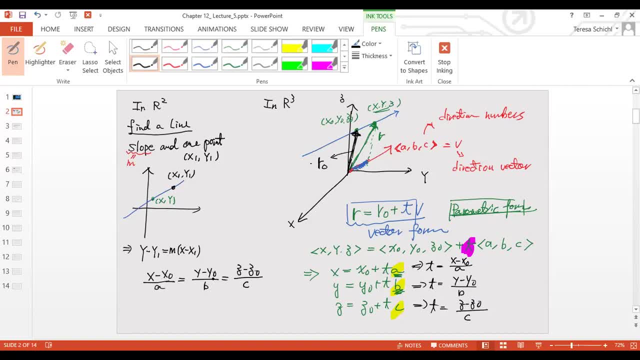 y minus y zero to the b, y minus y. zero to the b and is equal z minus, and is equal z minus z and is equal z minus z zero to the c, and what do we call zero to the c and what do we call zero to the c? and what do we call these ones here, these forms? 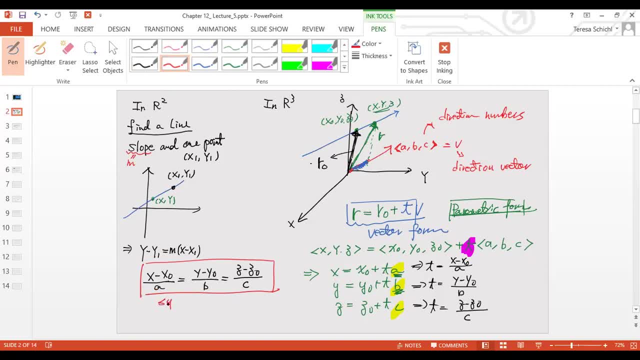 these ones here, these forms, these ones here, these forms here. we call this a symmetric form. okay, so we have a three way. okay, so we have a three way. okay, so we have a three way to write a you know a line. to write a. you know a line. 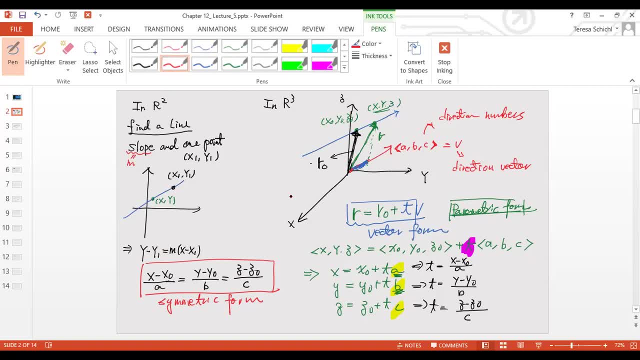 to write a. you know a line in the: what in the r3s here, all right in the. what in the r3s here, all right in the. what in the r3s here, all right. so the, so, the, so, the. i said the concept of what is pretty. 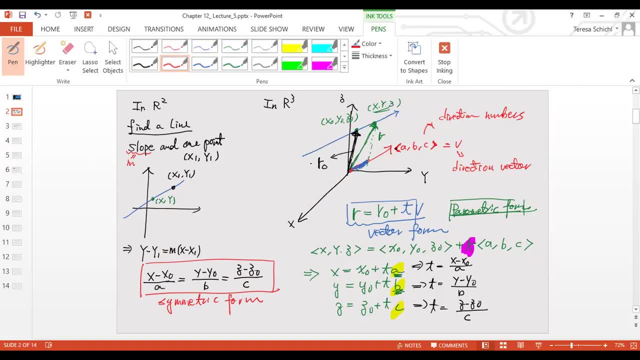 i said the concept of what is pretty. i said the concept of what is pretty, similar right. so you need to pass in similar right. so you need to pass in similar right, so you need to pass in through a point, through a point, through a point. then you need to know which direction is. 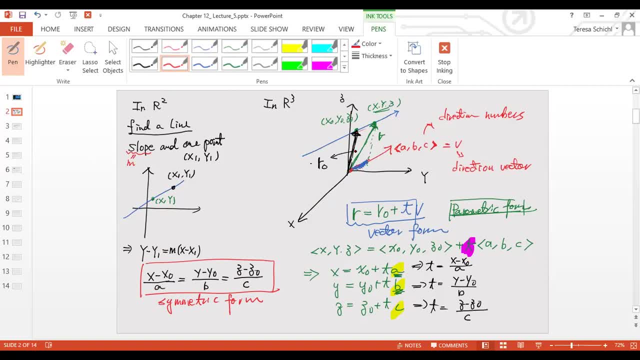 then you need to know which direction is, then you need to know which direction is here, then we just use here, then we just use here, then we just use our- you know the vectors addition, our, you know the vectors addition, our, you know the vectors addition to find the lines here. okay, so take a. 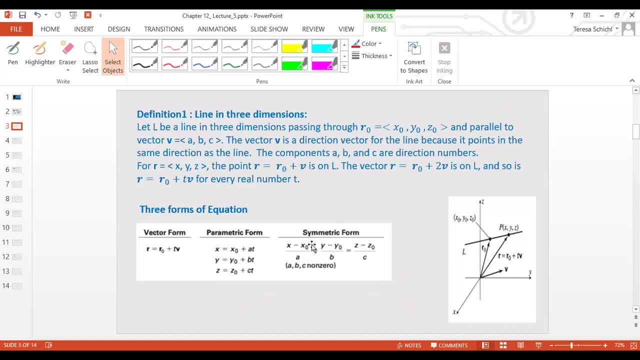 to find the lines here? okay, so take a. to find the lines here? okay, so take a. look at that's what is the definition. look at that's what is the definition. look at that's what is the definition. we just went through here, i hope you. we just went through here, i hope you. 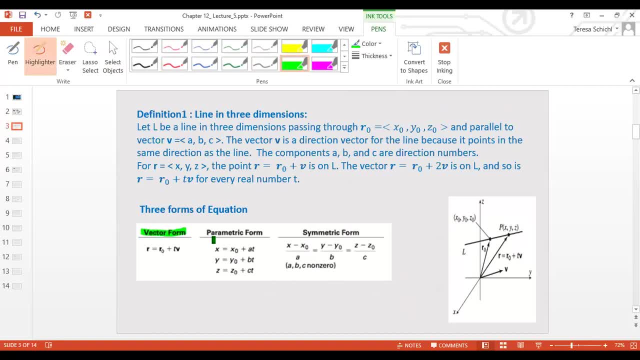 we just went through here. i hope you understand, understand, understand and so remember. we have the vectors and so remember. we have the vectors and so remember. we have the vectors form: parametrics form and the symmetrics form. parametrics form and the symmetrics form. parametrics form and the symmetrics form. 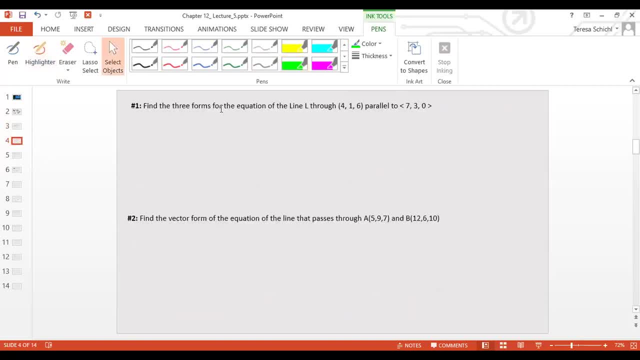 form- form. all right, okay, so now let's take a look. all right, okay, so now let's take a look. all right, okay, so now let's take a look. let's take a look at how do we do the. let's take a look at how do we do the. 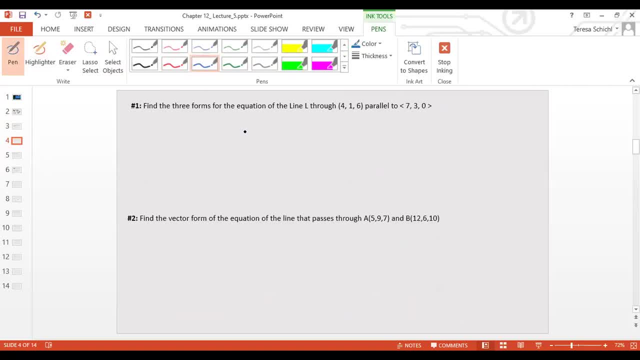 let's take a look at how do we do the problems here, problems here, problems here. so they said number one is here. find the. so they said number one is here, find the. so they said number one is here. find the three form, three form, three form for the line. this line goes through. 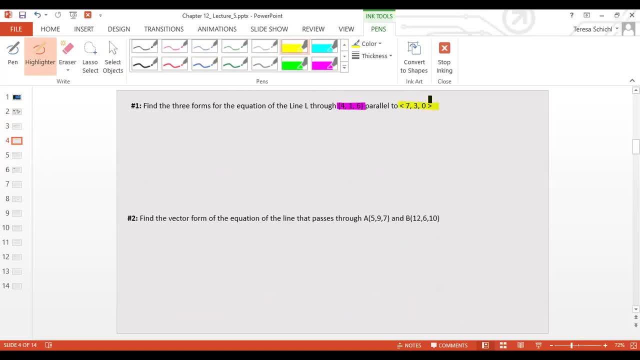 for the line this line goes through. for the line, this line goes through: four one, six, four one, six, four one, six, and this line is parallel to seven three, and this line is parallel to seven three, and this line is parallel to seven three, zero, zero, zero. so seven three, zero. this is a what? 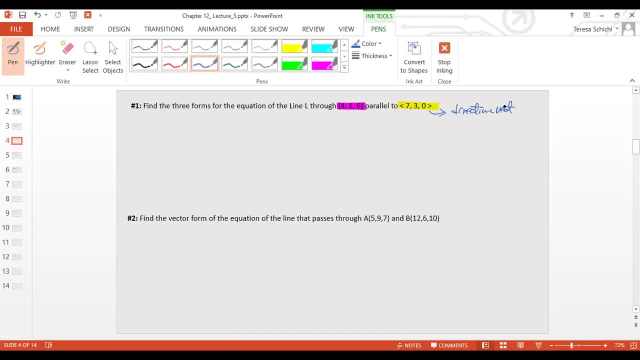 so seven three zero, this is a what. so seven three zero, this is a what. this is my direction. vectors, right, this is my direction. vectors, right, this is my direction. vectors, right, okay. so by the vectors form, so let's okay. so by the vectors form, so let's. 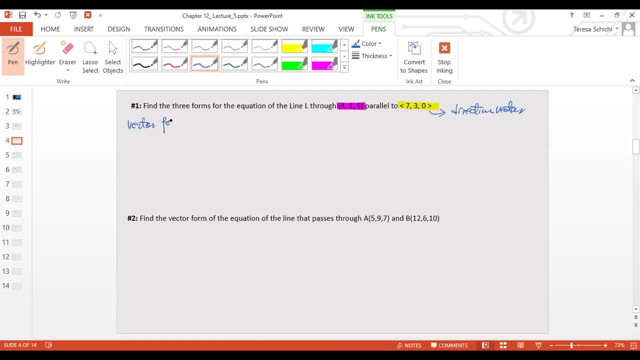 okay, so by the vectors form. so let's take a look at vectors form. take a look at vectors form. take a look at vectors form. okay, vectors form is the r. okay, vectors form is the r. okay, vectors form is the r. right, so is r is equal to the r zero. 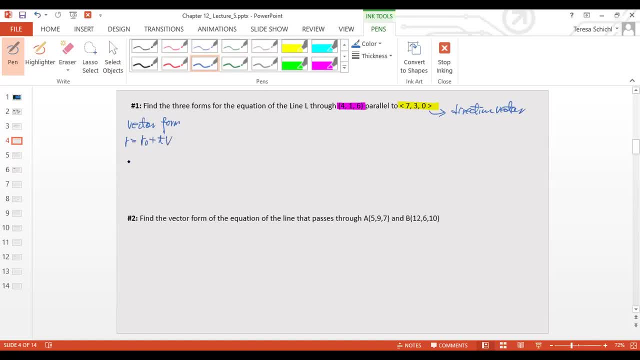 right? so is r is equal to the r zero, right? so is r is equal to the r zero plus t v plus t v plus t v. so that's why we say the r zero is what. so that's why we say the r zero is what. 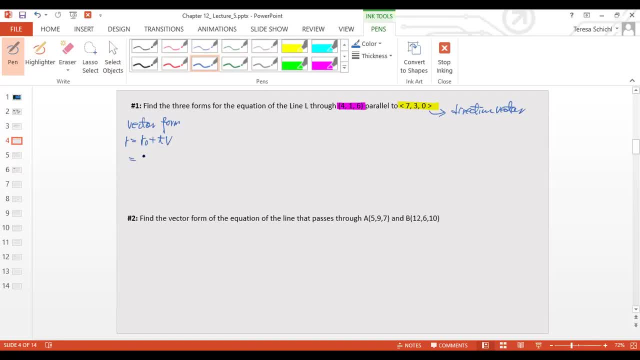 so that's why we say: the r zero is what? so? the r zero is four one six, so the r zero is four one six. so the r zero is four one six, right, so the four one six right. so the four one six right. so the four one six. so plus t t times the v. so this vector 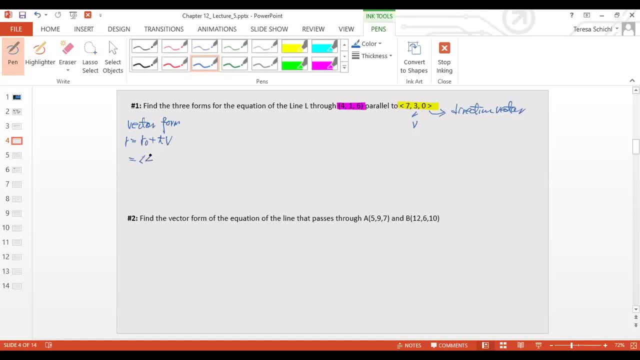 so plus t t times the v, so this vector. so plus t t times the v, so this vector is the v vectors right. is the v vectors right. is the v vectors right. so it will be what is four plus what. so it will be what is four plus what. 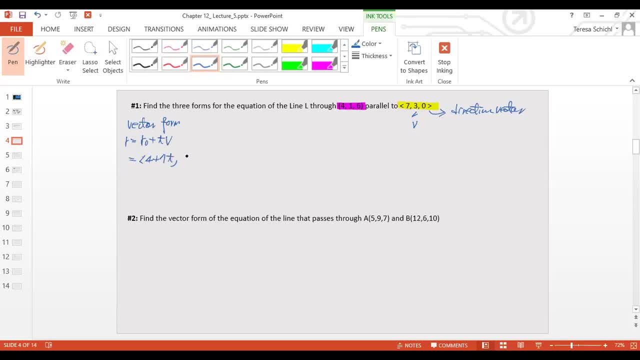 so it will be what is four plus what seven, seven, seven t and t and t, and now here is one plus, now here is one plus, now here is one plus what three t, what three t, what three t and what six is right and what six is right. 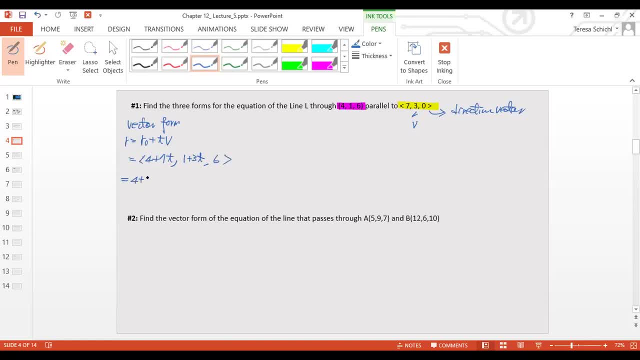 and what six is right, so that's a vector. so if you want you, so that's a vector. so if you want you, so that's a vector. so if you want, you can write it as a four plus, can write it as a four plus, can write it as a four plus seven t. 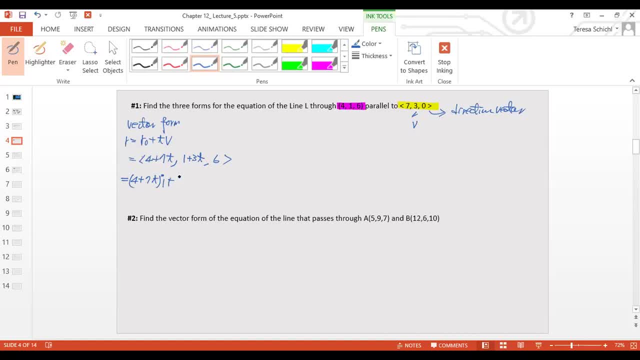 seven t, seven t, the i, the i, the i plus one plus three t plus one plus three t plus one plus three t a j, a, j, a j plus six k. so that's what we talk about, plus six k. so that's what we talk about. 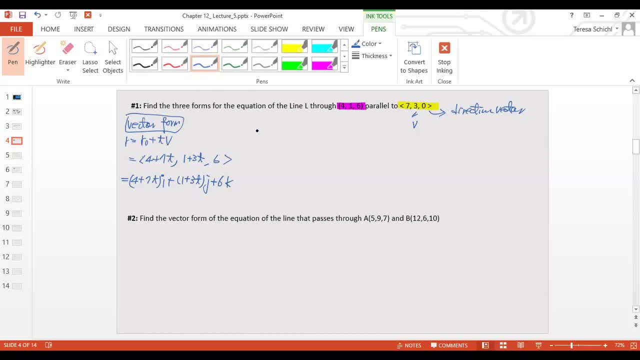 plus six k. so that's what we talk about: is the vectors term. is the vectors term? is the vectors term. now, let's take a look at the parametric. now let's take a look at the parametric. now let's take a look at the parametric term. 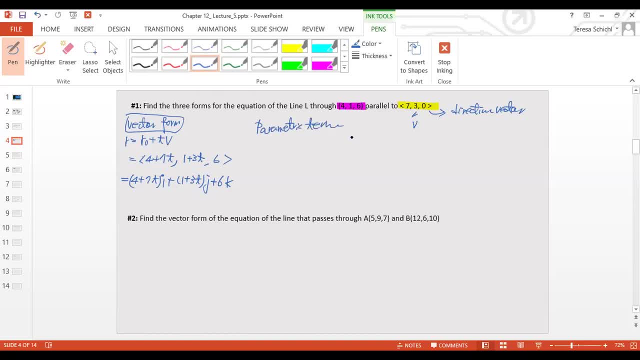 okay, so the parametric terms here: so it's okay. so the parametric terms here: so it's okay. so the parametric terms here, so it's x, y, z's right, so x is equal to x. x, y, z's right, so x is equal to x. 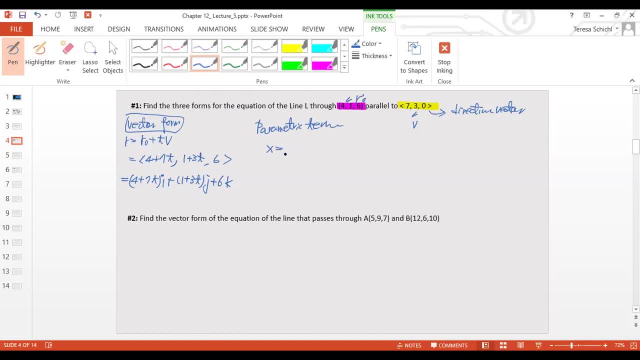 x, y, z's right. so x is equal to x zero. so this is the r zero, so that's zero. so this is the r zero, so that's zero. so this is the r zero. so that's the point that it goes through. so it's the point that it goes through, so it's. 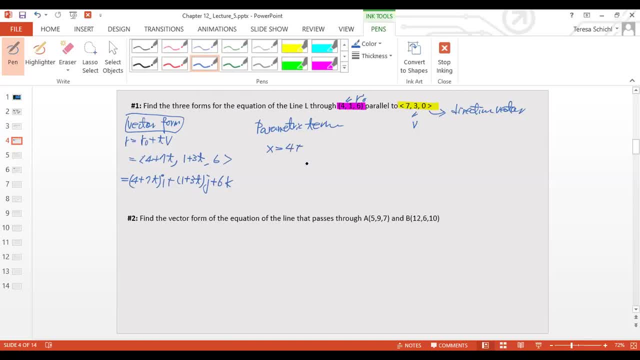 the point that it goes through. so it's a four plus what? four plus a four plus what. four plus a four plus what. four plus seventeen, seventeen, seventeen, and the y is equal to what and the y is equal to what, and the y is equal to what. one plus what. three t. 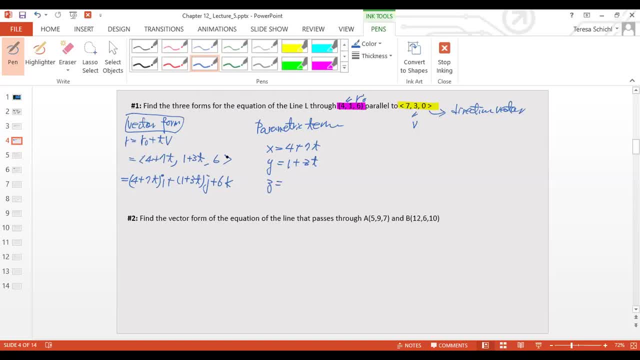 one plus what three t. one plus what three t. and what is this here z? and what is this here z? and what is this here? z is just what six, right? so it's is just what six, right? so it's is just what six, right, so it's six. okay, now let's do the symmetric. 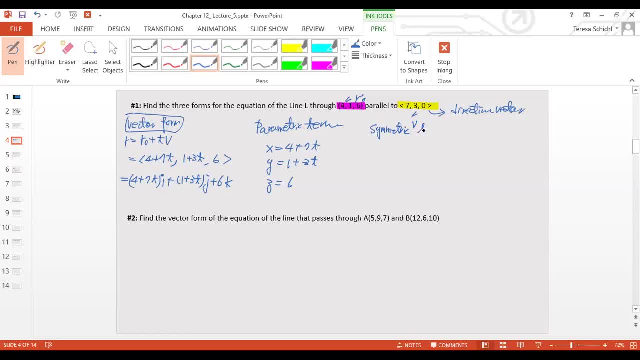 six. okay, now let's do the symmetric six. okay, now let's do the symmetric term. okay, so the symmetric term. so i know the x. okay, so the symmetric term. so i know the x. okay, so the symmetric term, so i know the x, minus minus, minus, minus four. 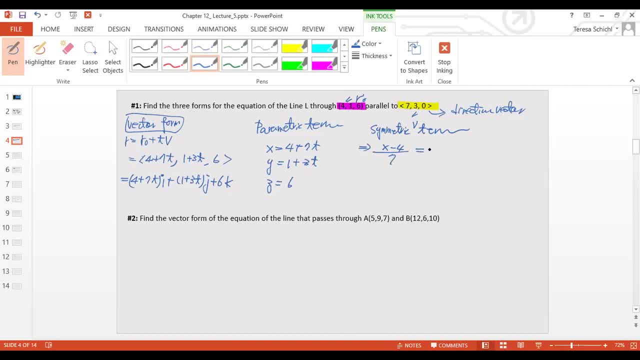 four. four over seven is equal to over seven is equal to over seven, is equal to y minus one over three, y minus one over three, y minus one over three. but z doesn't have a t, so i need to. but z doesn't have a t, so i need to. 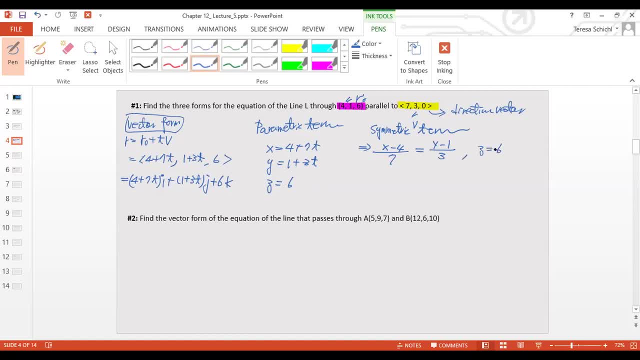 but z doesn't have a t, so i need to write a z, write a z, write a z for two sixths here. so this problem for two sixths here, so this problem for two sixths here, so this problem here is, here is here, is kind of very mechanical problem, show you. 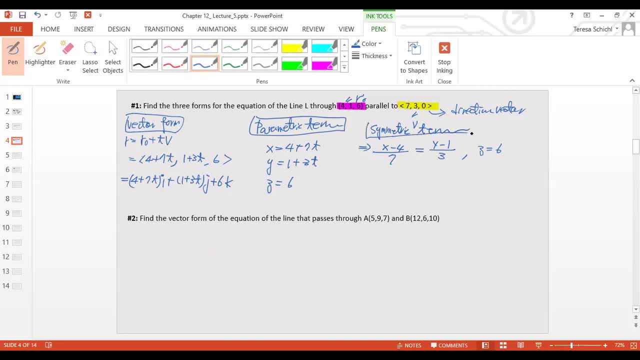 kind of very mechanical problem. show you kind of very mechanical problem. show you how do we write the line. how do we write the line, how do we write the line? by using a three different, by using a three different, by using a three different form to write our line in r3. 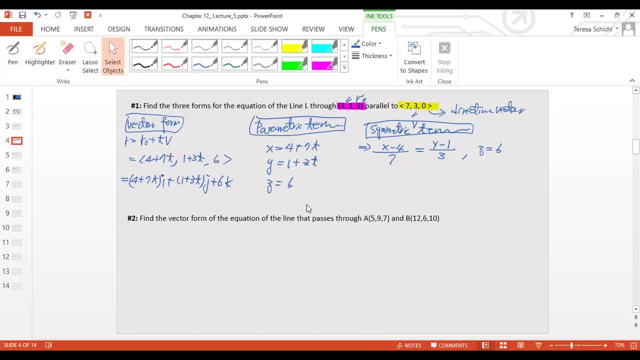 form to write our line in r3 form. to write our line in r3: a lot of people. they have um, a lot of people. they have um, a lot of people. they have um, i think a lot of people, it's kind of like, i think a lot of people, it's kind of like. 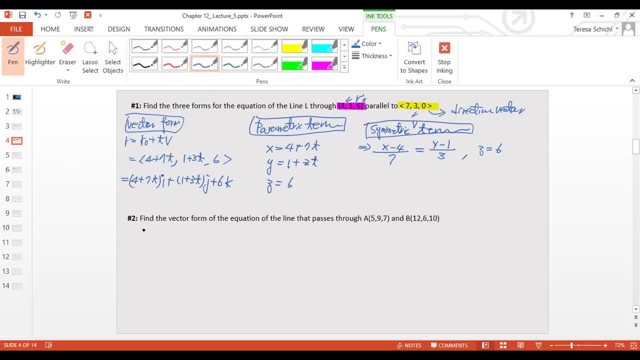 i think a lot of people. it's kind of like very difficult to visualize it. you know, very difficult to visualize it. you know very difficult to visualize it. you know so what? so what? so what? this is a line all right. so yeah, it is. this is a line all right. so yeah, it is. 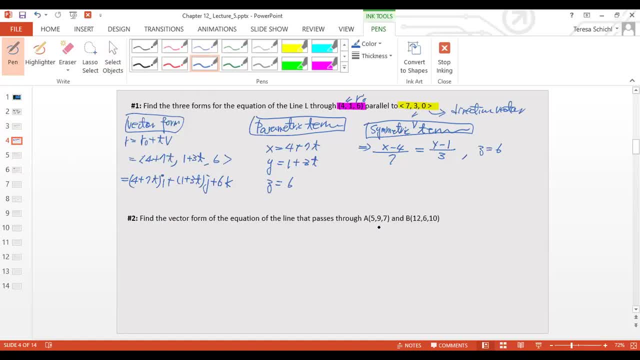 this is a line, all right. so yeah, it is alliance here, alliance here, alliance here- okay, so now let's take a look here. so i okay, so now let's take a look here. so i okay, so now let's take a look here. so i want to find. 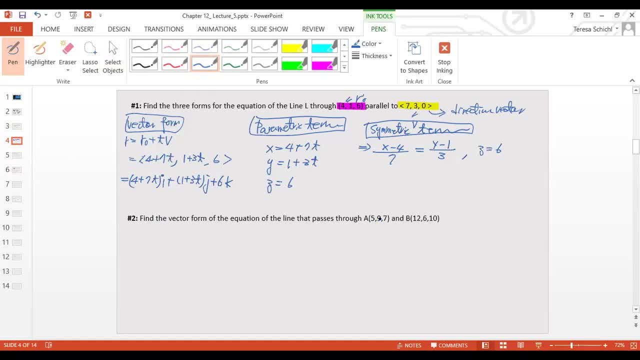 want to find, want to find the vectors. you know the i want to find the vectors. you know the i want to find the vectors. you know the i want to find the vectors form, the vectors form, the vectors form, to the line passing through two points, to the line passing through two points. 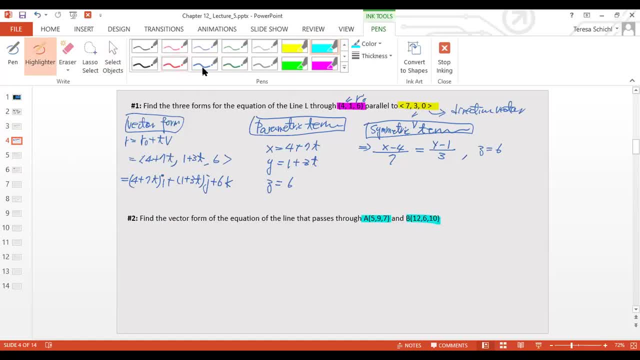 to the line passing through two points here right now. they give you these two here right now. they give you these two here right now. they give you these two points, points, points. all right. so how do i do it so, if you all right? so how do i do it? so, if you? 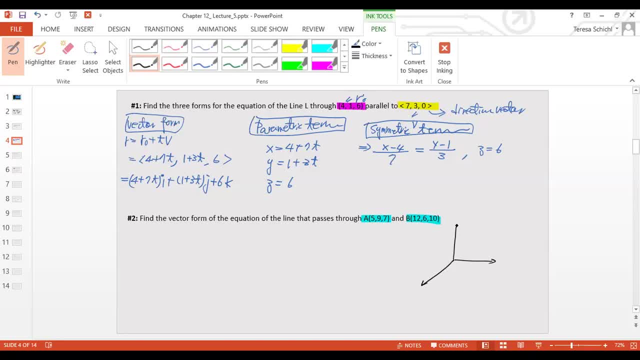 all right. so how do i do it? so if you take a look at this one, take a look at this one, take a look at this one here right. so that means if you have a here right. so that means if you have a here right. so that means if you have a pointer number ones here, pointer number. 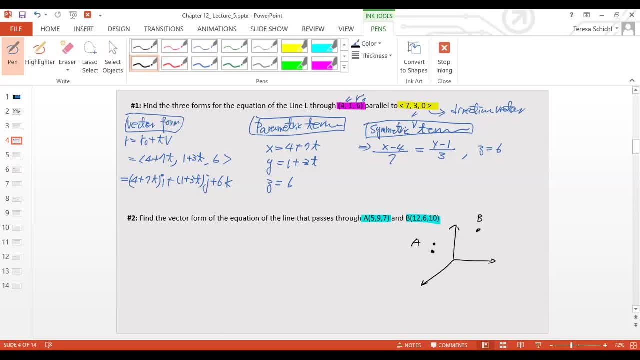 pointer number ones here, pointer number. pointer number ones here. pointer number two here: i don't know this is right. or two here, i don't know this is right. or two here, i don't know this is right or not, but this is, for example, this is a b's. 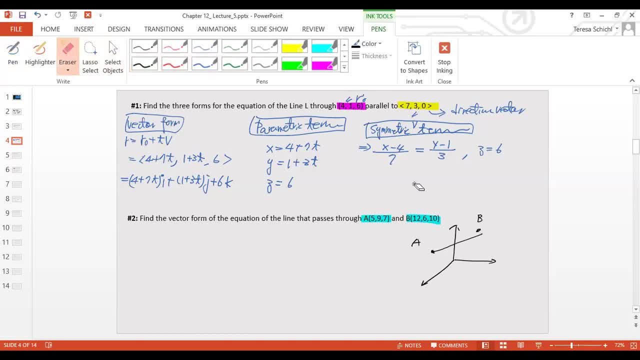 not, but this is, for example, this is a b's, not, but this is, for example, this is a b's, right, right, right, so you have two points here. so you have two points here. so you have two points here. okay, so you have two points. okay, so you have two points. 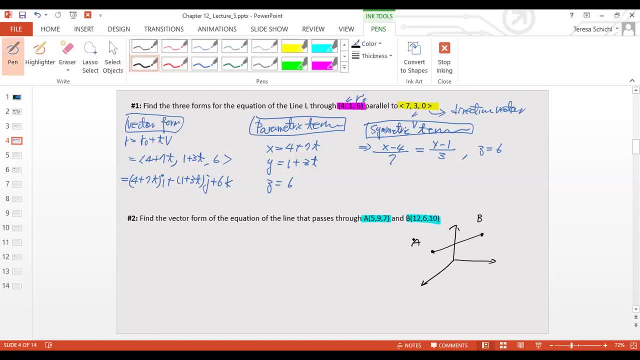 okay. so you have two points: all right and now all right, and now all right and now okay. so remember why we need to have a. okay, so remember why we need to have a. okay, so remember why we need to have a. so this is a line goes through these two. 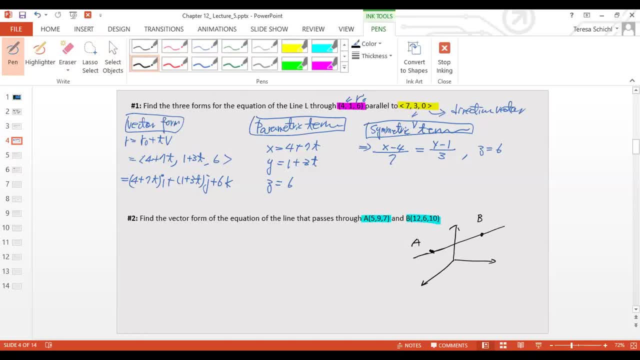 so this is a line goes through these two. so this is a line goes through these two, point point, point point a and the point b is here. so point a and the point b is here. so point a and the point b is here. so the first thing is here. remember from the: 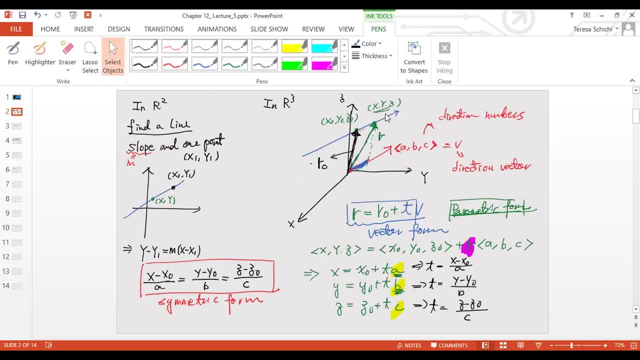 the first thing is here. remember from the. the first thing is here. remember from the. here we need to have x y z's right, so x. here we need to have x y z's right, so x. here we need to have x y z's right, so x y z. 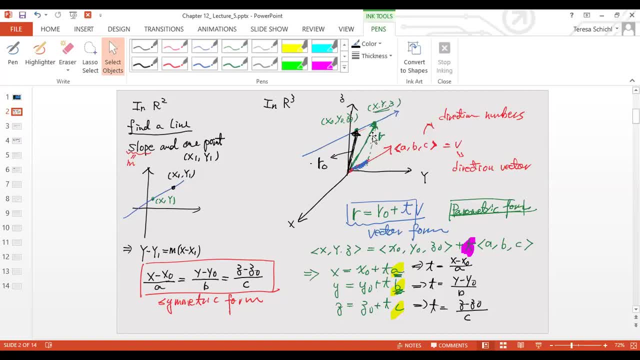 y z y z. that's the ending general. you know so. that's the ending general. you know so. that's the ending general. you know so, this, this, this, you know this one's here, right so it. you know this one's here, right so it. you know this one's here, right so it has to be parallel. 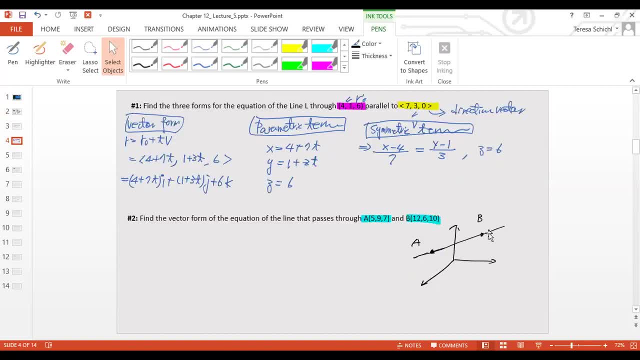 has to be parallel, has to be parallel. you will need to find the directional. you will need to find the directional, you will need to find the directional vector. so first let's try to find the vector. so first let's try to find the vector. so first let's try to find the vector of a b's here, right, so the 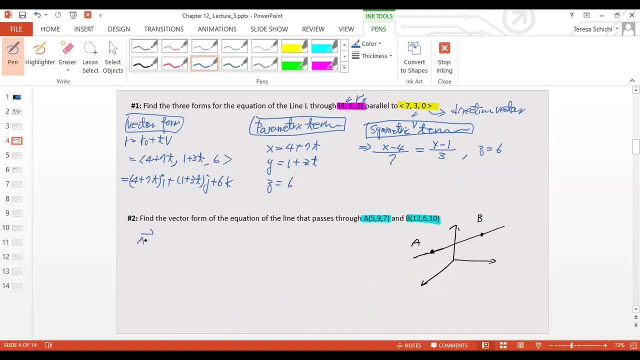 vector of a- b's here, right, so the vector of a- b's here, right, so the so the a b here. so we say that this so the a b here. so we say that this so the a- b here. so we say that this vector from the a to b's right, all right. 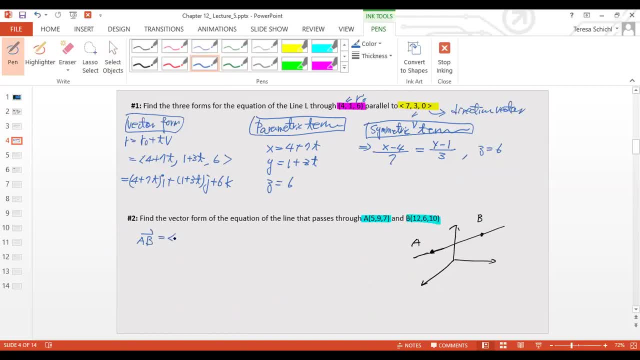 vector from the a to b's right- all right. vector from the a to b's right- all right. so a to b, so a to b. so a to b, it will be 12 minus 5 and 6 minus 9 and and 6 minus 9 and. 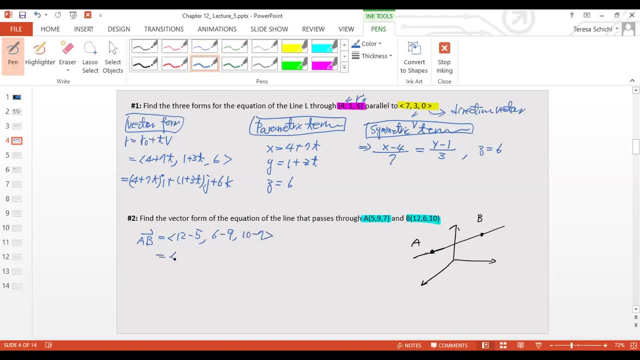 and 6 minus 9 and 10 minus 7, 10 minus 7, 10 minus 7. what is here? have a seven negative three. what is here? have a seven negative three. what is here? have a seven negative three and the what and the what. 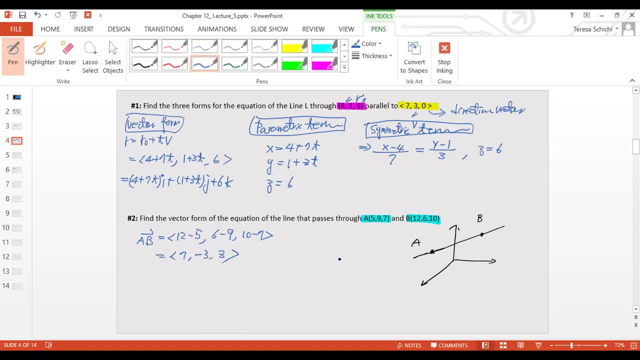 and the what and the three. it's right, seven negative and the three. it's right, seven negative and the three. it's right, seven negative. three and the three. what is this one? three and the three. what is this one? three and the three? what is this one? because this one we just did is this: we. 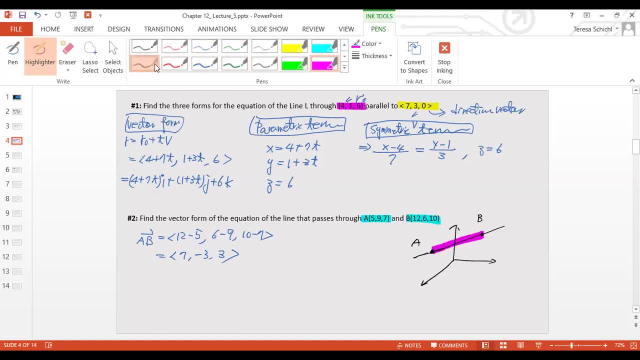 because this one we just did is this we? because this one we just did is this: we did a, did a, did a. we did this segment right. we said this. we did this segment right. we said this. we did this segment right. we said this is the is the. 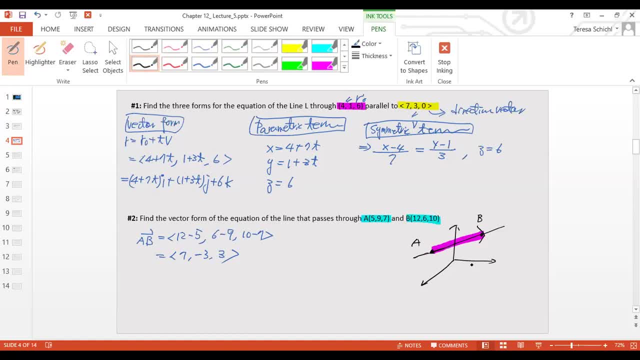 is the vector right. we did this segment, so i vector right. we did this segment, so i vector right, we did this segment. so i know, know, know from previous. so i know what is here my from previous. so i know what is here my from previous, so i know what is here my directional vector. 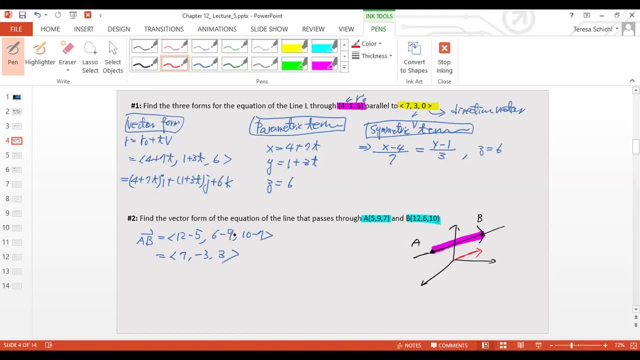 directional vector. directional vector has to be parallel to here. so now after i have directional vector, so now after i have directional vector, so now after i have directional vector, then i can use the vector form, so i will. then i can use the vector form, so i will. 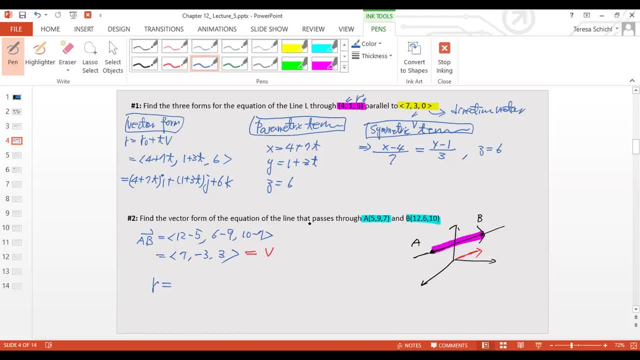 then i can use the vector form. so i will just say, just say, just say: r is equal to the r zero, r is equal to the r zero, r is equal to the r zero. i can use my r zero is a five nine. i can use my r zero is a five nine. 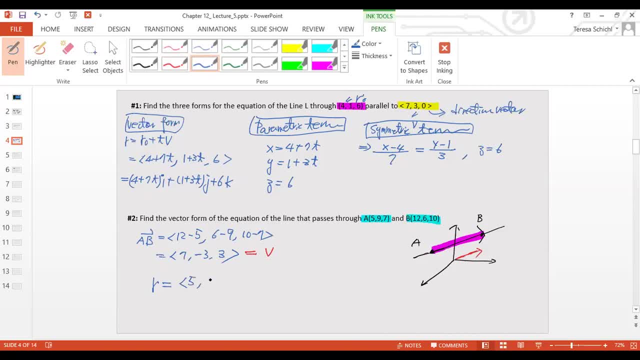 i can use my r: zero is a five, nine, seven, right? so i say: is it a five, seven, right? so i say: is it a five, seven, right? so i say: is it a five, nine, seven, nine, seven, nine, seven? then plus the t, then plus the t. 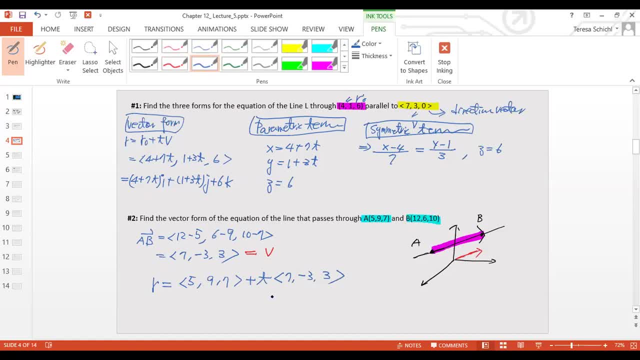 then, plus the t right, seven negative three and the seventh right, seven negative three and the seventh right, seven negative three and the seventh here, here, here, right. so that's what you know, that is right. so that's what you know, that is right. so that's what you know, that is our lines here, right? so remember. 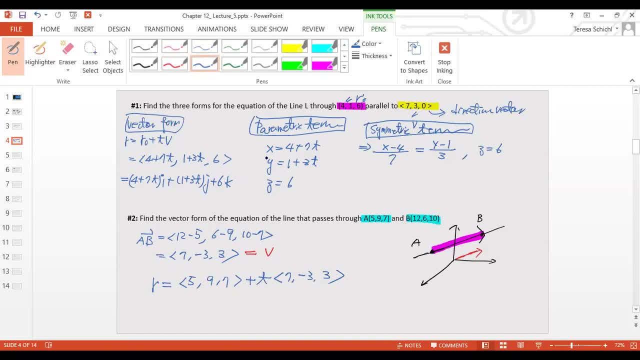 our lines here, right? so remember our lines here, right. so remember, just like in r2 a line we need to have, just like in r2 a line we need to have, just like in r2 a line. we need to have a point and we need to have a direction. 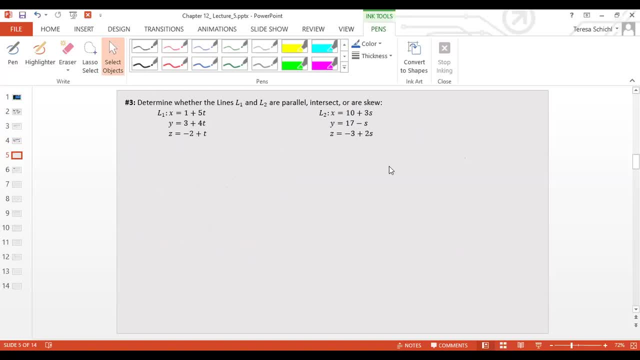 a point and we need to have a direction. a point and we need to have a direction right, so we need to know where it goes right. so we need to know where it goes right. so we need to know where it goes. okay, now let's take a look. 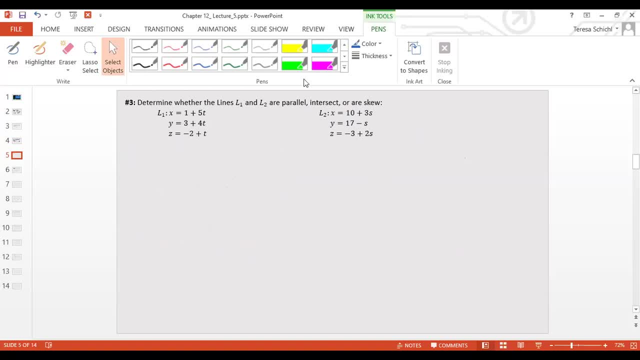 okay, now let's take a look. okay, now let's take a look here, right so determine whether the here right so determine whether the here right so determine whether the line, line, line l1 and l2, they are parallel intersect. l1 and l2, they are parallel intersect. 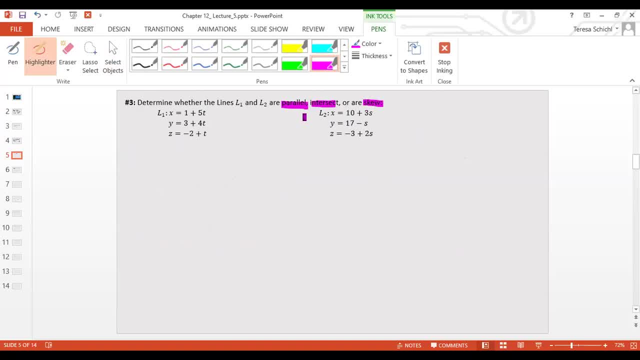 l1 and l2, they are parallel. intersect: or skew, okay, skew. or skew, okay skew. or skew, okay, skew. that means they will never intersect. that means they will never intersect. that means they will never intersect. and uh, but they are not, apparently. and uh, but they are not apparently. 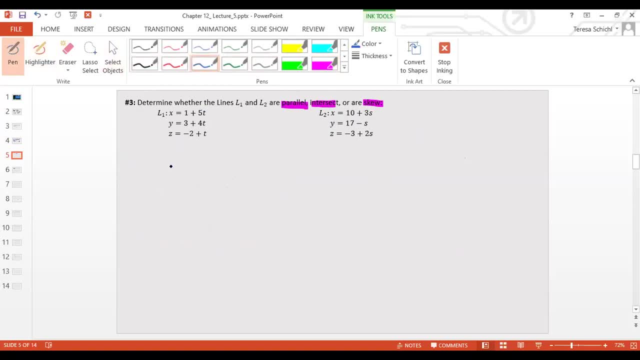 and uh, but they are not, apparently, okay. so now let's take a look here. the okay. so now let's take a look here. the okay. so now let's take a look here. the first ones here, the first ones here, the first ones here, the nine ones, right. so remember, this is a 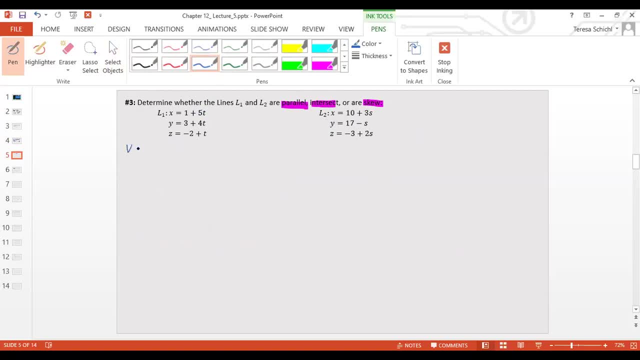 nine ones, right? so remember, this is a nine ones, right? so remember, this is a parametric, parametric, parametric form. so what is my v? or this is my form? so what is my v? or this is my form? so what is my v? or this is my direction? 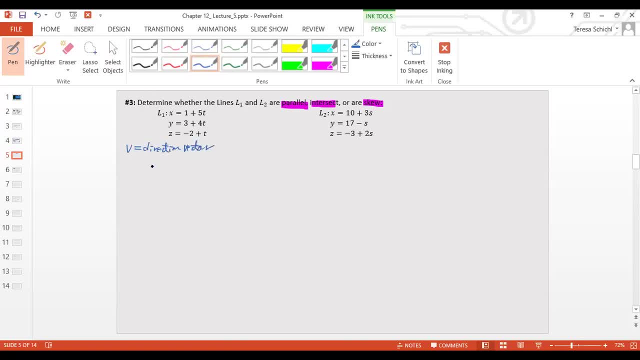 direction, direction. so this is my direction vector. so where is so? this is my direction vector. so where is so? this is my direction vector. so where is this line, the direction? go. this line, the direction, go, this line, the direction, go. so go what five, so go what five. 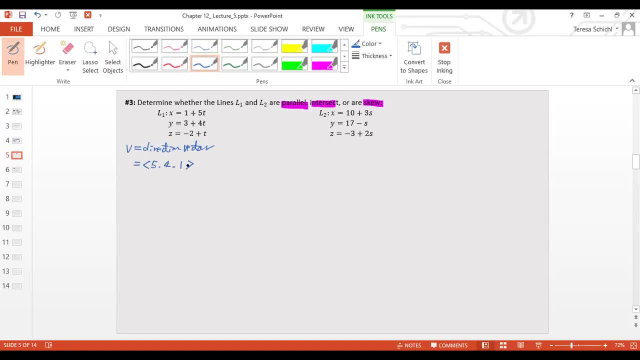 so go what? five, four, four, four, and the water: five, four and one. and the water: five, four and one, and the water: five, four and one. it's right, it's right, it's right. and what is this one's this go? this is. and what is this one's this go? this is: 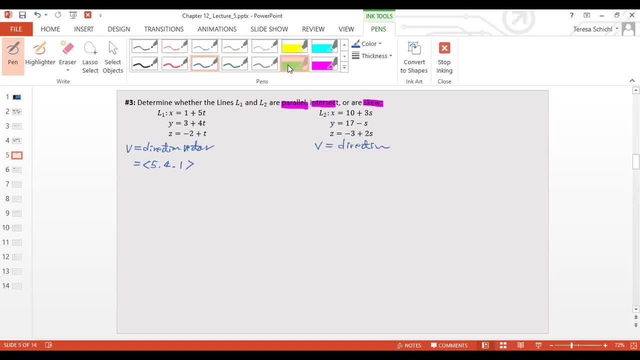 and what is this one's this go. this is the, the, the okay. so the direction. so this is the okay. so the direction. so this is the okay. so the direction. so this is the five four one. so this is the direction. five four one, so this is the direction. 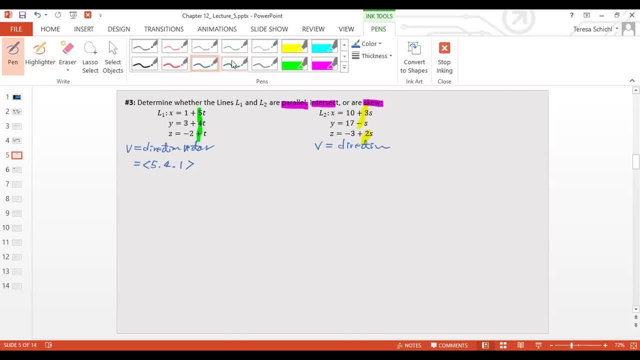 five, four, one. so this is the direction right. so for here, this one is the right. so for here, this one is the right. so for here, this one is: the vector is three, vector is three, vector is three: negative one and two. so if you compare negative one and two, so if you compare, 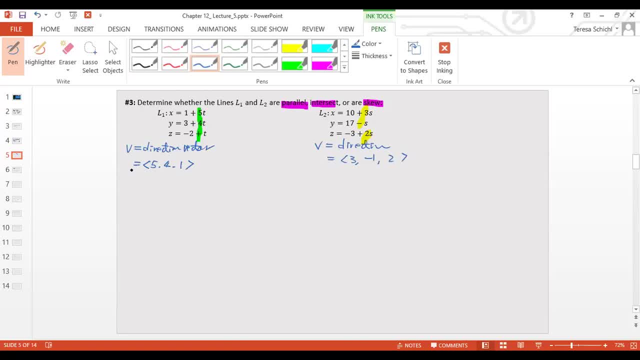 negative, one and two. so if you compare these two direction vectors, these two direction vectors, these two direction vectors, layer right and they are. they are not layer right and they are. they are not layer right and they are. they are not multiplied by a constant. so i said v1. 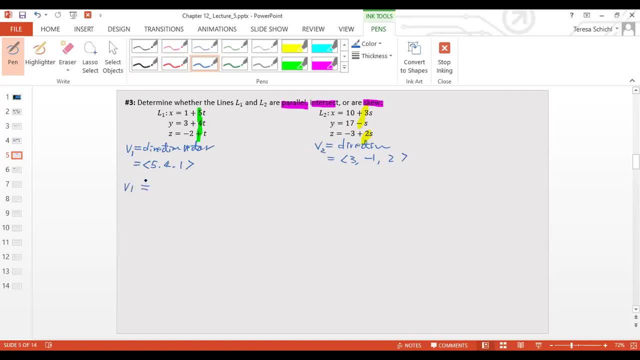 multiplied by a constant, so i said v1. multiplied by a constant, so i said v1, v2 right. so v y is not equal to v2 right. so v y is not equal to v2 right. so v y is not equal to a constant times v2. 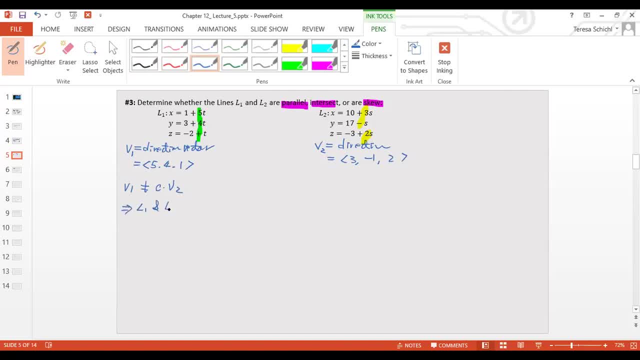 a constant times v2, a constant times v2- right. so now i know l1 and l2 right. so now i know l1 and l2 right. so now i know l1 and l2 is not what parallel is, not what parallel is not what parallel- right, so they are not a parallel, see. 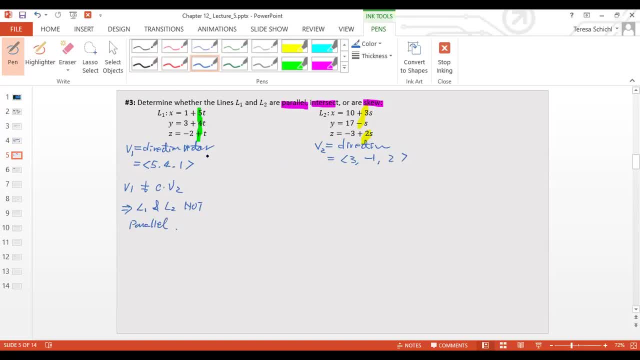 right, so they are not a parallel. see, right, so they are not a parallel. see here, here, here, okay, so now let's see. so the first. okay, so now let's see. so the first, okay, so now let's see. so the first things we come to, things we come to. 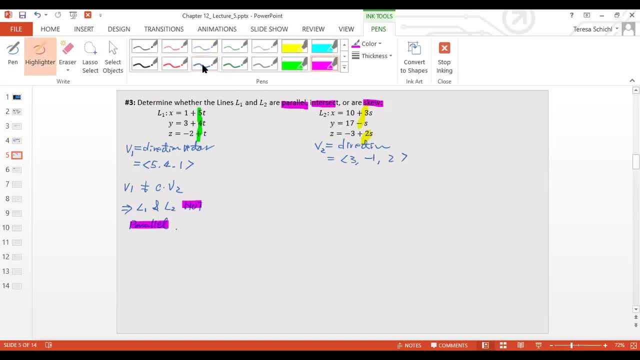 things we come to conclusion is not parallel. okay, so the conclusion is not parallel. okay, so the conclusion is not parallel. okay, so the next things we want to see is next things we want to see is next things we want to see is they are intersect or not. what do we? 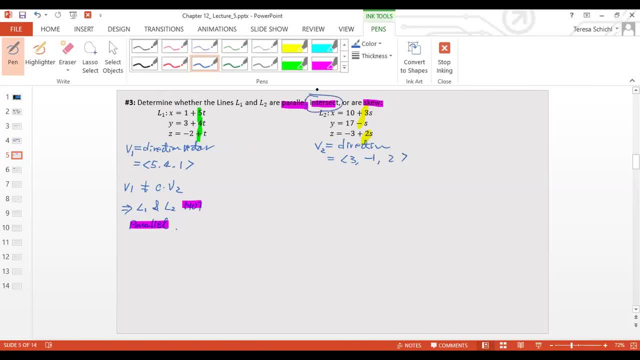 they are intersect or not. what do we? they are intersect or not. what do we mean? intersect, mean, intersect, mean, intersect. you know, just like in the geometry, we you know, just like in the geometry, we you know, just like in the geometry, we say: l line 1 equal to line 2. that means: say l line 1 equal to line 2, that means say l line 1 equal to line 2. that means x need to be equal to the x and y. x need to be equal to the x and y. x need to be equal to the x and y equal to y. 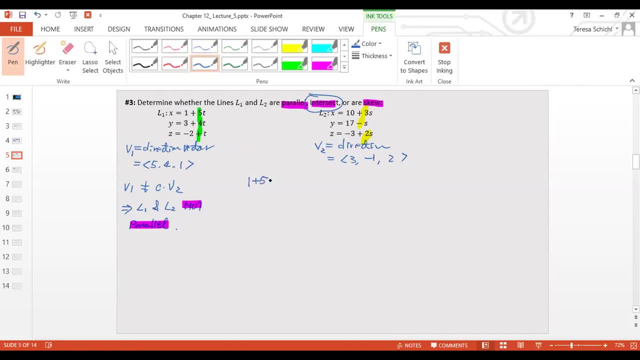 equal to y. equal to y right. so that means one plus right. so that means one plus right. so that means one plus five t. this has to be equal to the 10 five t. this has to be equal to the 10 five t. this has to be equal to the 10 plus. 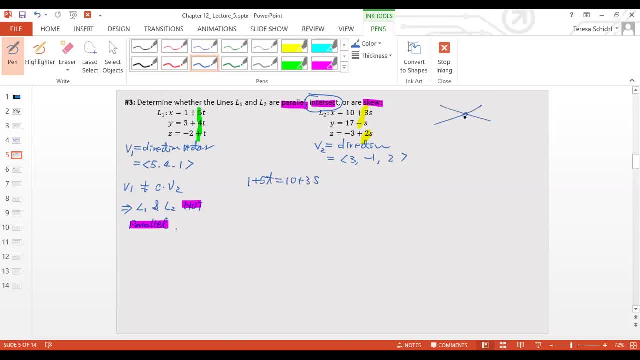 plus plus three s right, because the two lines three s right, because the two lines three s right, because the two lines intersect. that means intersect. that means intersect. that means the x and the x going to, you know the, the x and the x going to, you know the. 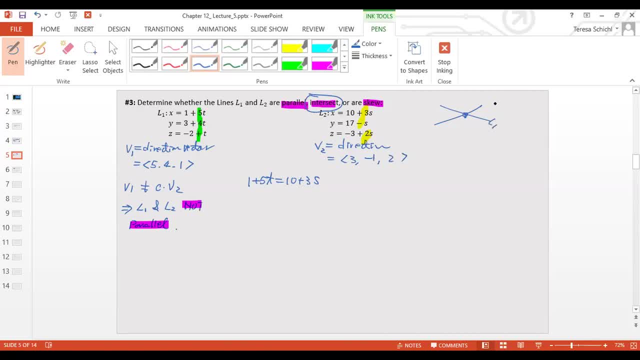 the x and the x going to, you know, the x y z on the this line, which have to be x y z on the this line, which have to be x y z on the this line, which have to be equal to the x y z on the other line. equal to the x y z on the other line. equal to the x y z on the other line right. so x is one plus five t in one right. so x is one plus five t in one right. so x is one plus five t in one line. 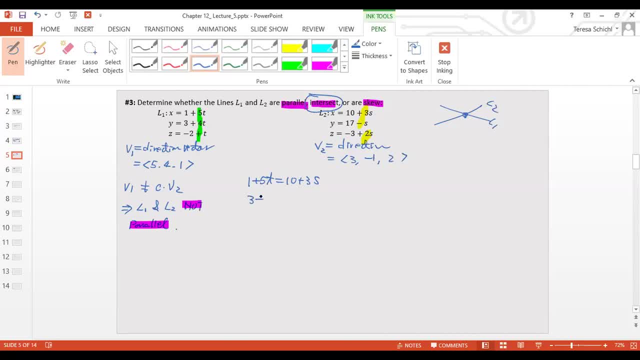 line line 10 plus 3s in another line. so this is a 10 plus 3s. in another line. so this is a 10 plus 3s in another line. so this is a 3 plus 3 plus 3 plus 4t has to be equal to the 17 minus. 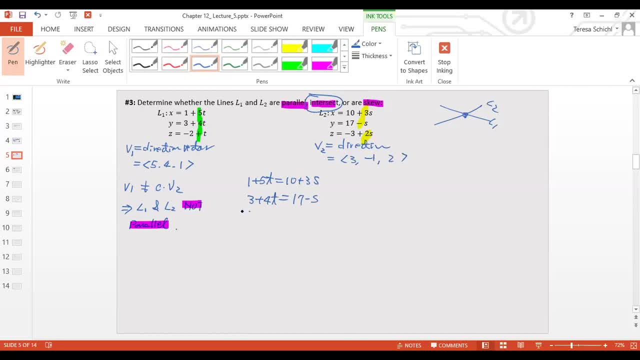 4t has to be equal to the 17 minus 4t has to be equal to the 17 minus s. and now s and now s and now. this one here is negative: 2 plus t. this one here is negative: 2 plus t. 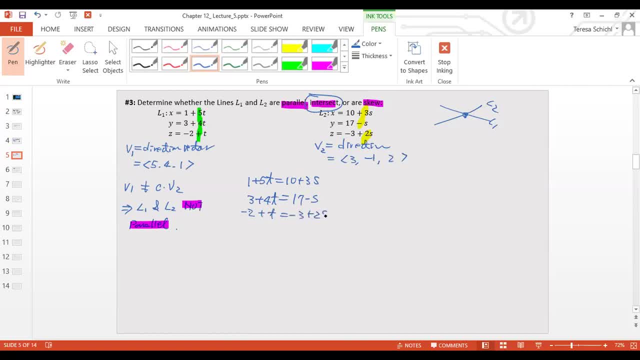 this one here is negative: 2 plus t has equal to the negative. 3 plus 2s. has equal to the negative. 3 plus 2s has equal to the negative 3 plus 2s here. okay, so now let's try to solve so. 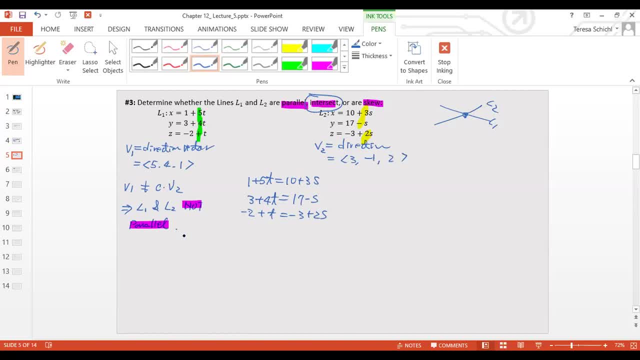 here, okay, so now let's try to solve. so here, okay, so now let's try to solve. so basically, we want to see, basically we want to see, basically we want to see this layer solution. so we want to solve this layer solution, so we want to solve. 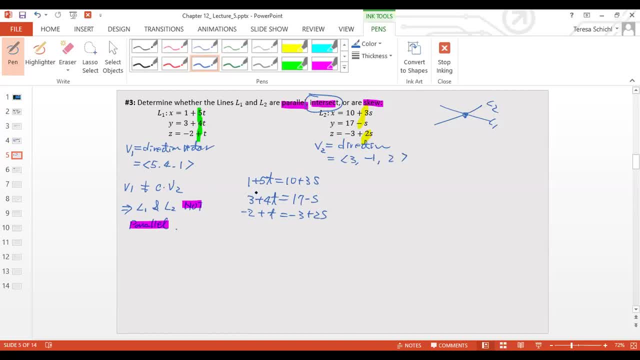 this layer solution. so we want to solve for s and t. so what i need to do here for s and t, so what i need to do here for s and t, so what i need to do here, i guess i solve the system of equations. i guess i solve the system of equations. 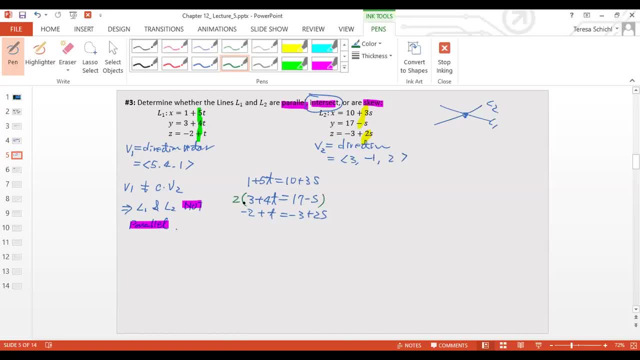 i guess i solve the system of equations. so i times, so i times. so i times what i times two on both sides, then add what i times two on both sides, then add what i times two on both sides, then add to the, to the, to the, you know, then add to the third. 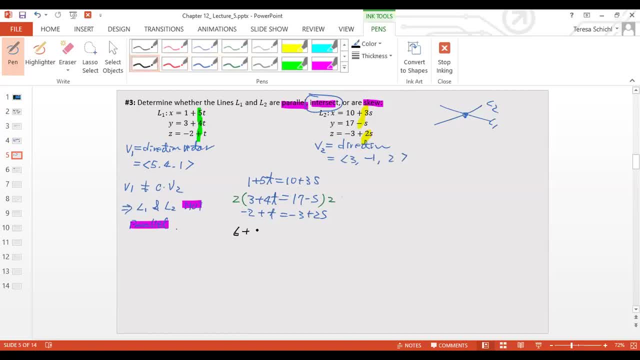 you know, then add to the third. you know, then add to the third: equation, so times two. so this is equation, so times two. so this is equation, so times two. so this is six plus 80 equal to the 34. six plus 80 equal to the 34. 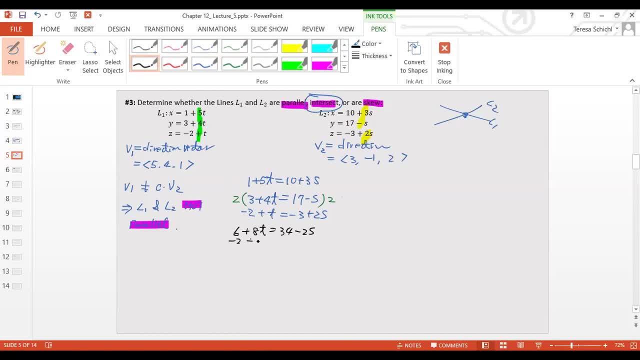 six plus 80, equal to the 34 minus 2s. now i add to the third minus 2s. now i add to the third minus 2s. now i add to the third equation. so this is negative 3 minus equation. so this is negative 3 minus. 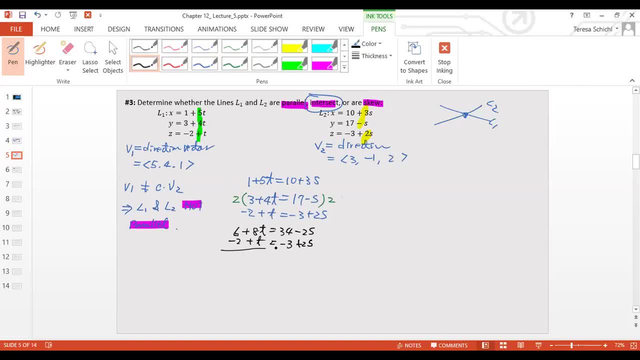 equation. so this is negative: 3 minus 2s plus 2s, 2s plus 2s, 2s plus 2s. so this one cancels right. so this one cancels right. so this one cancels, right, okay. so this one cancel. 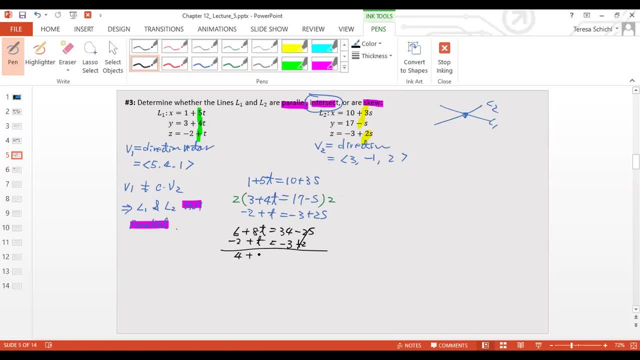 okay, so this one cancel. okay, so this one cancel. and then this is the four plus, and then this is the four plus, and then this is the four plus: 90 is equal to 90 is equal to 90 is equal to what four plus? what four plus. 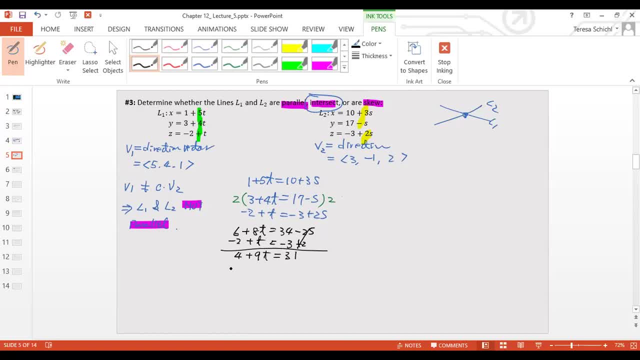 what? four plus 90 is equal to 31, 90 is equal to 31, 90 is equal to 31, so that means 90 equal to so that means 90 equal to. so that means 90 equal to 27, so t is equal to. 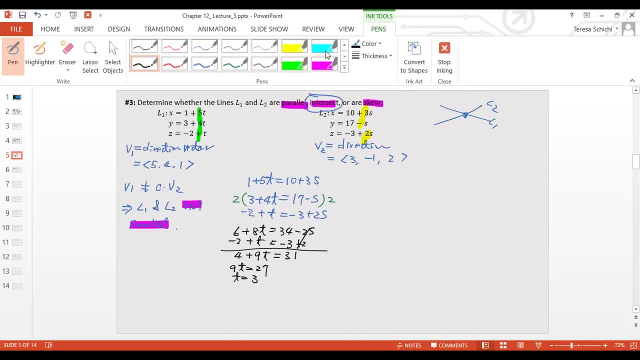 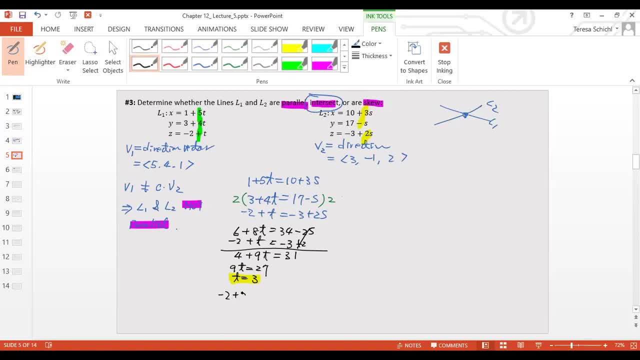 now, after i have a t equal to three, a now, after i have a t equal to three, a substitute to find the s substitute. to find the s substitute. to find the s. so negative, two plus three equal to the. so negative. two plus three equal to the. 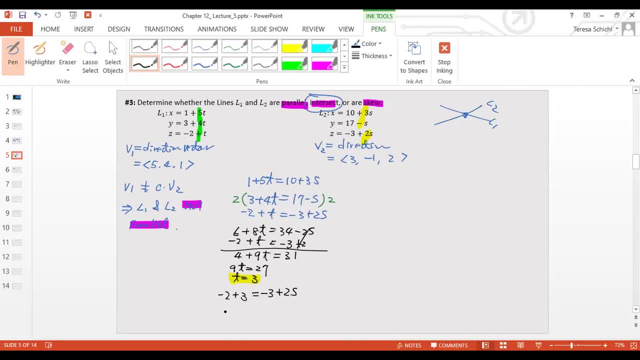 so negative two plus three equal to the negative three. negative three. negative three plus two s okay. so plus two s okay. so plus two s okay. so s equal to what solve, it s equal to what solve, it s equal to what solve it and s equal to. 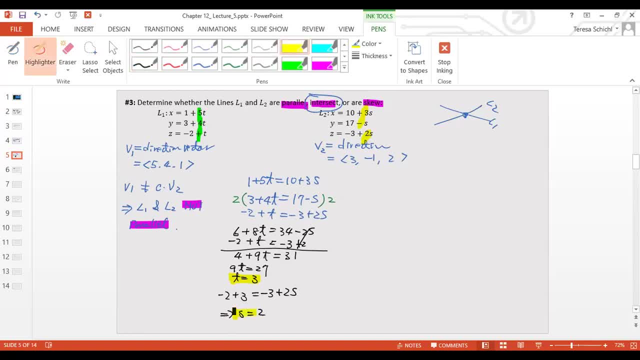 and s equal to and s equal to two. see here: okay, so two. see here: okay, so two. see here: okay, so okay, so s equal to two, so i use okay, so s equal to two, so i use: okay, so s equal to two, so i use these two equations. 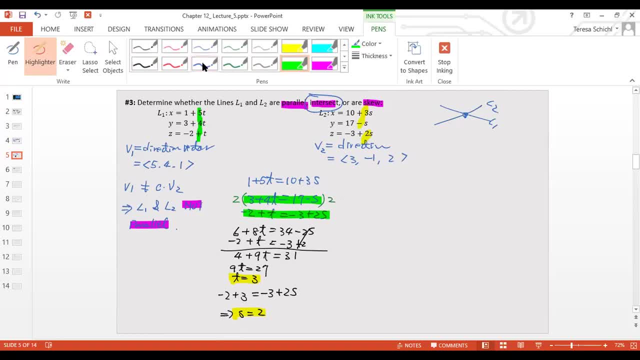 these two equations, these two equations to solve the s and t. now i need to. to solve the s and t, now i need to. to solve the s and t, now i need to substitute back to the first ones, right. substitute back to the first ones, right. substitute back to the first ones, right. so 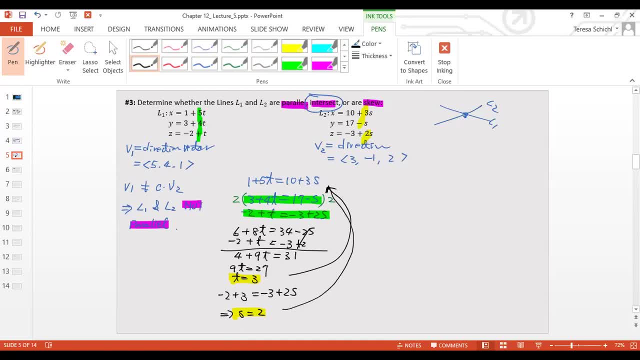 so so i need to substitute back to the first. i need to substitute back to the first, i need to substitute back to the first one to see one. to see one to see is true or not? so t, so it's one plus. is true or not? so t so it's one plus. 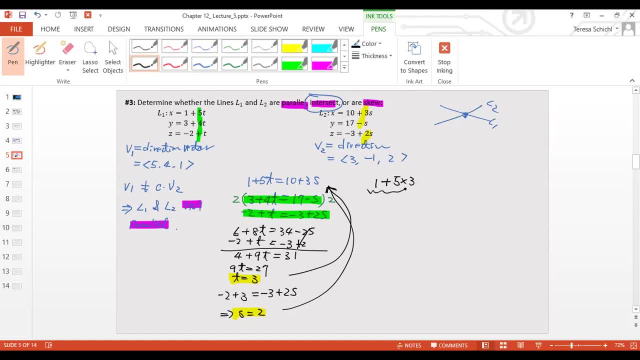 is true or not? so t. so it's one plus five times five times five times three. so the left hand side: this is 16, three. so the left hand side: this is 16: three. so the left hand side: this is 16 is this is equal to the right hand side. 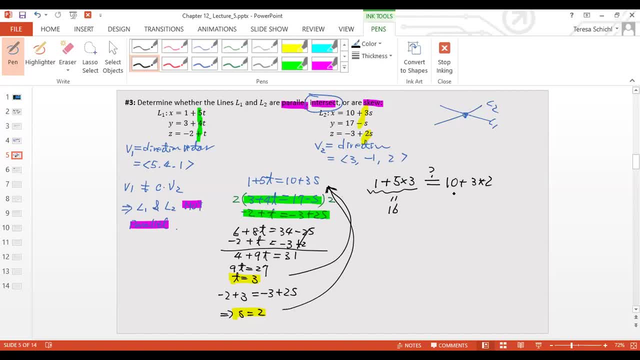 is this is equal to the right hand side, is this is equal to the right hand side. so it's a 10 plus. so it's a 10 plus. so it's a 10 plus three times two for every dollar. this is three times two for every dollar. this is: 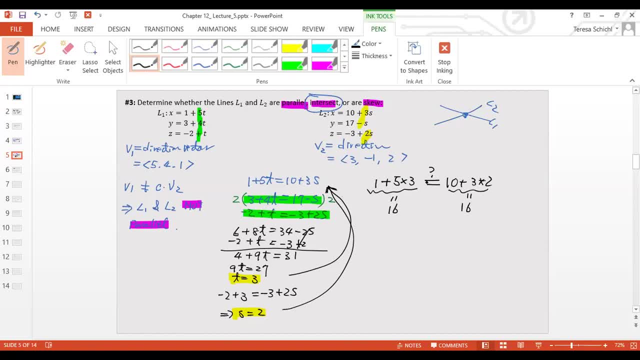 three times two for every dollar, this is equal to the 16.. equal to the 16.. equal to the 16.. so what is here? so yeah, they are. so what is here? so yeah, they are. so what is here? so yeah, they are equals, right. so when they are. 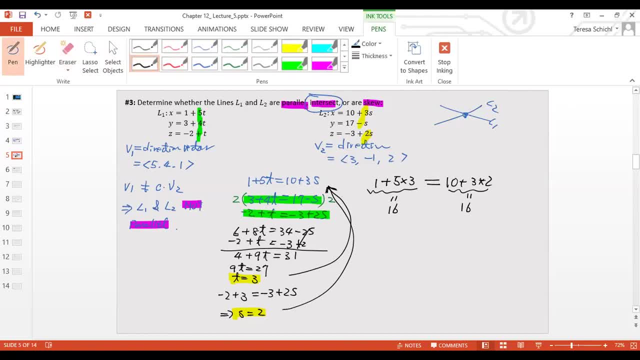 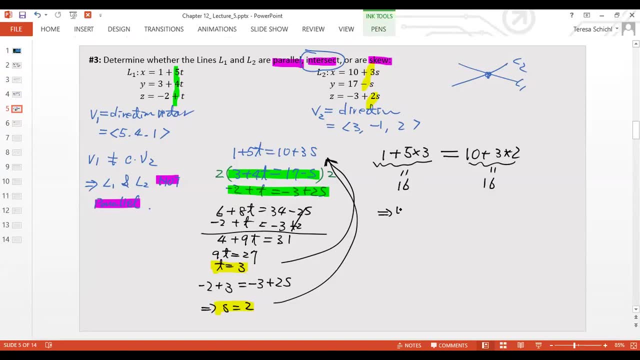 equals, right. so when they are equals, right. so when they are equals here, then what's that means equals here, then what's that means equals here, then what's that means here. so when they are equal, that means here. so when they are equal, that means here. so when they are equal, that means we have what, so that means we have a. 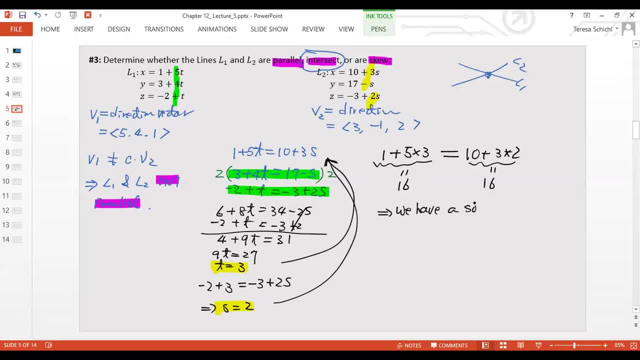 we have what, so that means we have a. we have what, so that means we have a solution, solution, solution. solution, that means this, that means this, that means this: two lines, so what two lines, so what two lines, so what? this two line intersect? all right, okay, so that means this two. 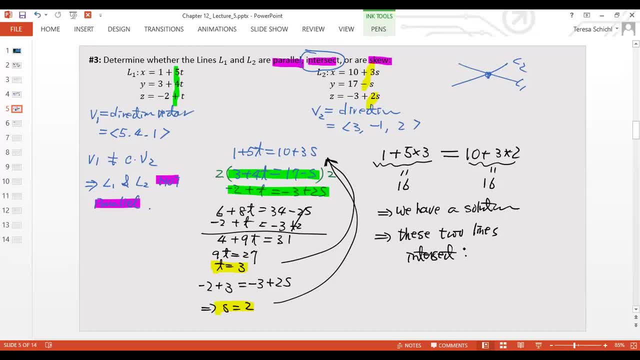 all right, okay, so that means this: two: all right, okay, so that means this: two: line intersect, line intersect, line intersect. you know, if they are not parallel, they you know, if they are not parallel, they you know. if they are not parallel, they not intersect, then they have to be. 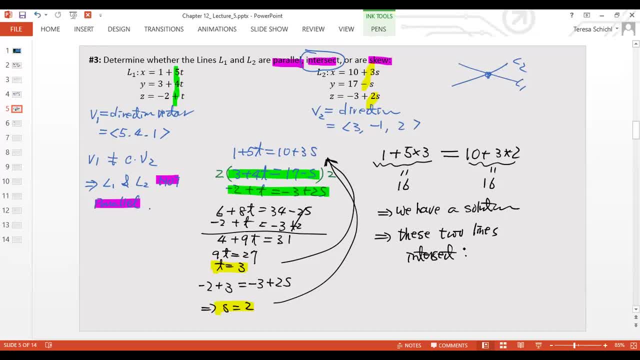 not intersect, then they have to be not intersect, then they have to be skewed here, skewed here, skewed here, okay. so now let's take a look at the okay. so now let's take a look at the okay. so now let's take a look at the next. 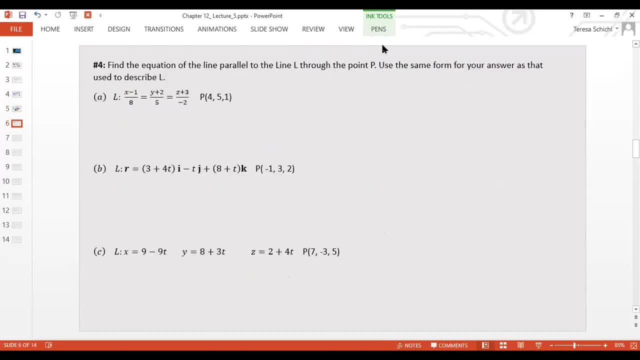 next, next, right. so find the equation of the line right. so find the equation of the line, right. so find the equation of the line, okay. okay, so find the equation of the line, okay. so this is a pretty mechanical also. so this is a pretty mechanical also. so this is a pretty mechanical also. i want to find the line parallel to the. 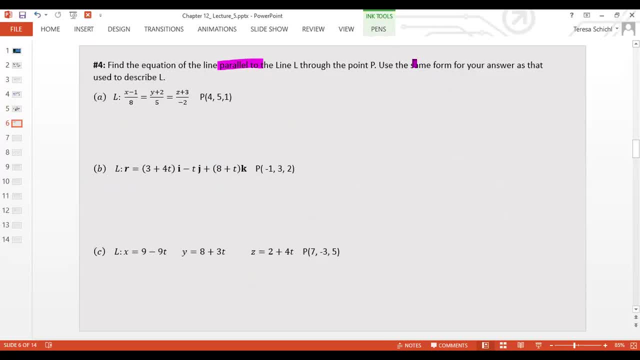 i want to find the line parallel to the. i want to find the line parallel to the line l, line l, line l, and through the given point, then use. and through the given point, then use and through the given point, then use the same form whatever, the same form whatever. 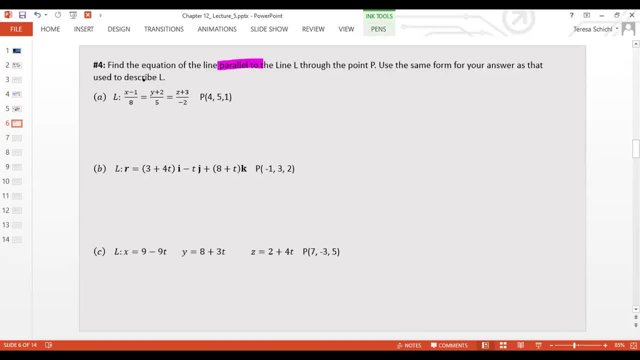 the same form, whatever you know the your problem given. so you know the your problem given. so you know the your problem given. so this is a parametric form, this is a parametric form, this is a parametric form. so i said to find the, then the passing. 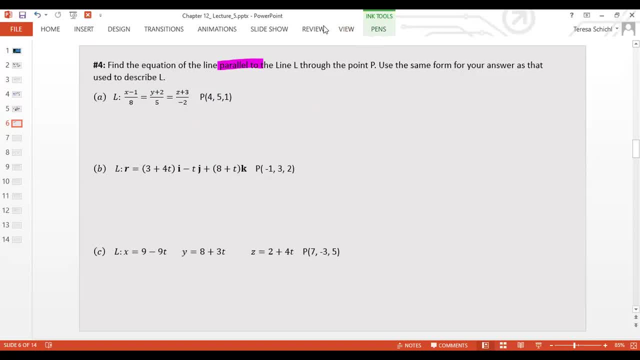 so i said to find the, then the passing. so i said to find the, then the passing, through this point, through this point, through this point. okay, so this is the easy right. so this: okay, so this is the easy right, so this is the easy right. so this: 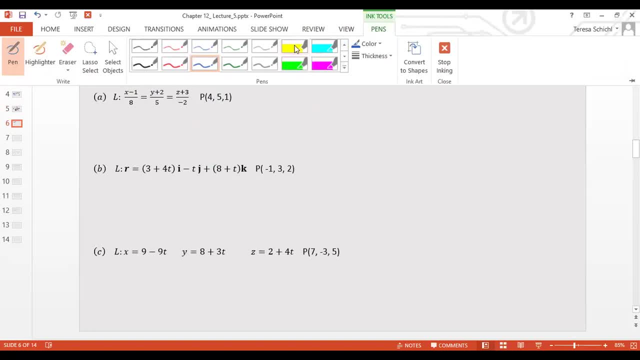 okay, so this is the easy right. so this one's here, one's here, one's here because so what? what are those number because? so what? what are those number because? so what? what are those number? how those are the directional number, how those are the directional number. 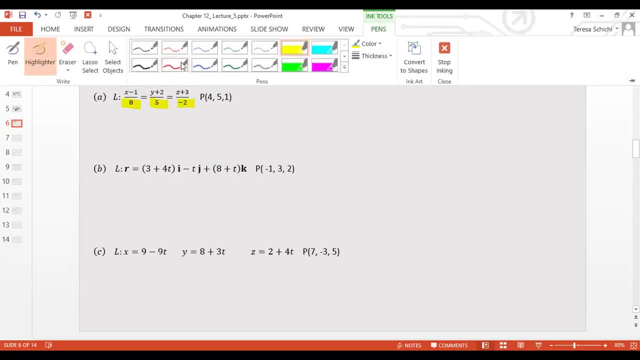 how those are the directional number. right directional vectors numbers here. right directional vectors numbers here. right directional vectors numbers here. so okay, so what is my answers here? so okay, so what is my answers here? so okay, so what is my answers here? so the a equal to five. 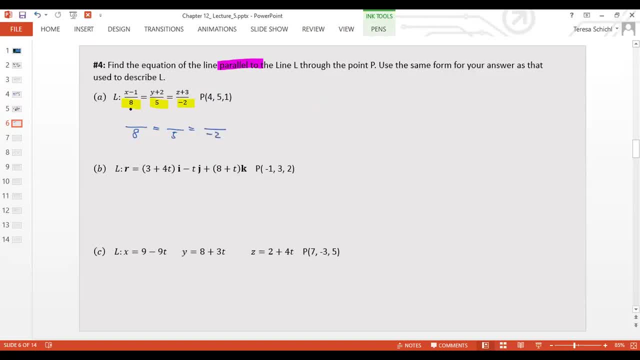 so the a equal to five, so the a equal to five, equal to negative two. because they are equal to negative two, because they are equal to negative two, because they are parallel, parallel, parallel. now it's passing through this specific. now it's passing through this specific, now it's passing through this specific point. so i just say x minus. 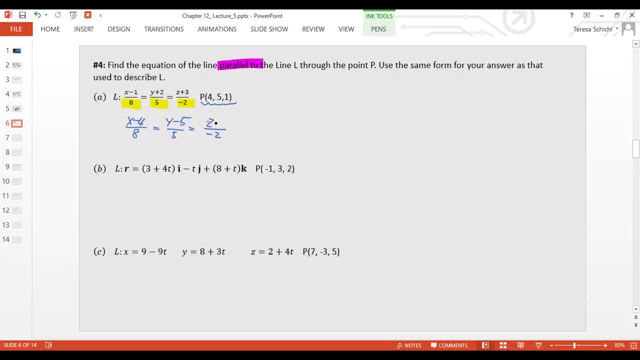 point. so i just say x minus point. so i just say x minus four, y minus five and z minus one. four, y minus five and z minus one. four, y minus five and z minus one. see here all right, okay. see here all right, okay. see here all right, okay. so now let's take a look the next ones. 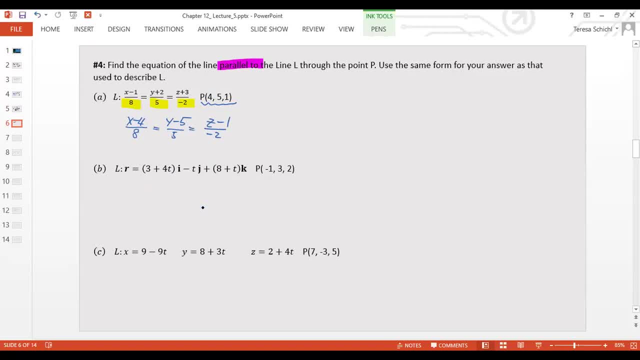 so now let's take a look the next ones. so now let's take a look the next ones here, right, so the next ones here. we say here: right, so the next ones here. we say here: right, so the next ones here. we say the r, the r. 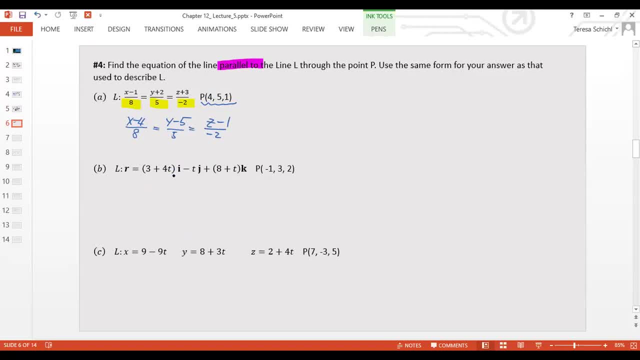 the r equal to three plus four t minus t, and equal to three plus four t minus t, and equal to three plus four t minus t, and the a plus t case here. the a plus t case here. the a plus t case here. okay, so let's see here where. 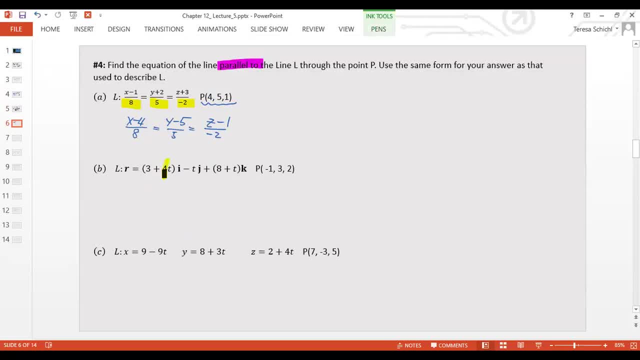 okay, so let's see here where. okay, so let's see here where is my, is my, is my directional vectors number? is this number directional vectors number? is this number directional vectors number? is this number right? so it's right, so it's right. so it's this number. and. 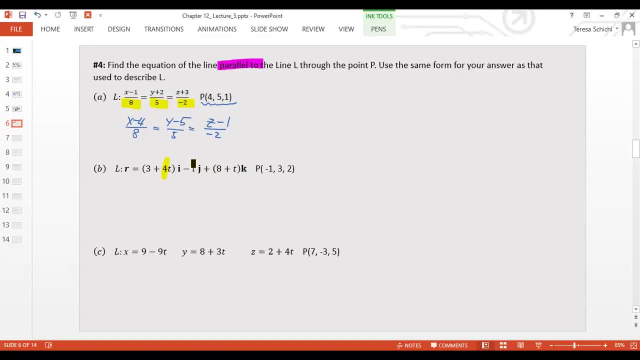 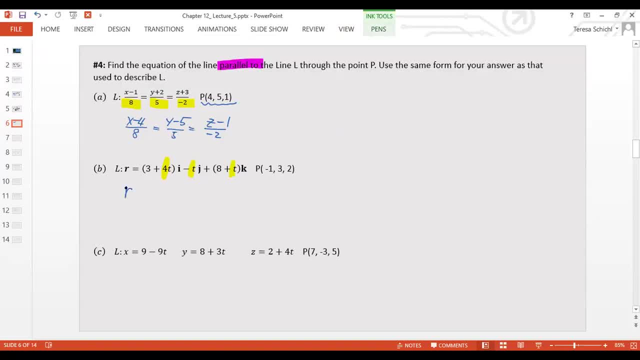 try to write it. try to write it, all right. so here, because it's the same, all right. so here, because it's the same, all right. so here, because it's the same way. so i know this way, so i know this way, so i know this r okay. so this is the up. let's say the. 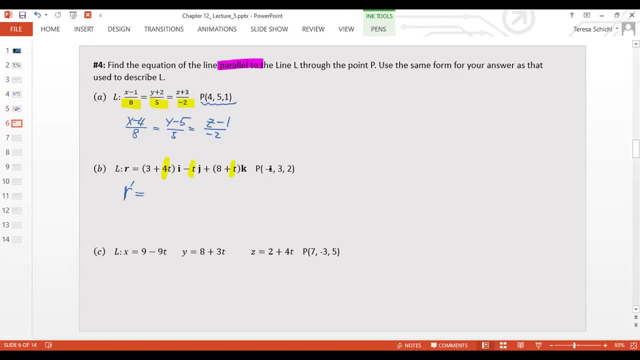 r. okay, so this is the up. let's say the r. okay, so this is the up. let's say the r prime is the one parallel to the r. r prime is the one parallel to the r. r prime is the one parallel to the r. so, instead of negative three, so we. 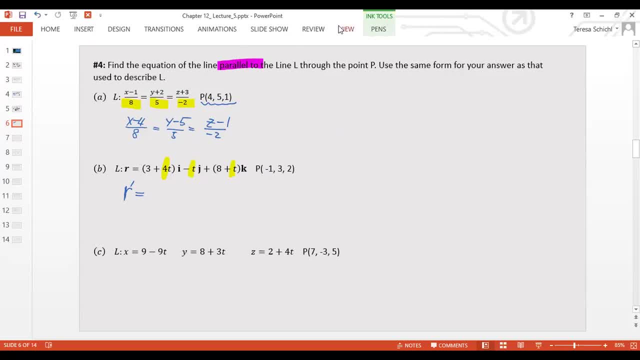 so instead of negative three, so we so, instead of negative three, so we notice, notice, notice those numbers like those numbers, like those numbers, like you know those numbers are what those you know those numbers are, what those you know those numbers are, what those are. the point are the point. 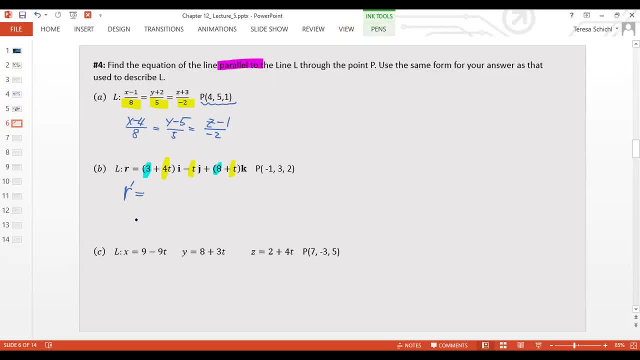 are the point: right, okay, so now let's try to write it. right okay, so now let's try to write it. right okay, so now let's try to write it. so what is here? we replace with a. so what is here? we replace with a. so what is here? we replace with a negative one. 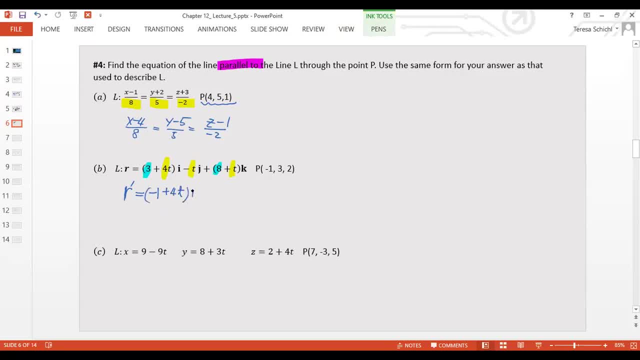 negative one. negative one plus 14, i plus 14, i plus 14, i right now. what is the second ones here right now? what is the second ones here right now? what is the second ones here is three, right, so it's three, but i have a. 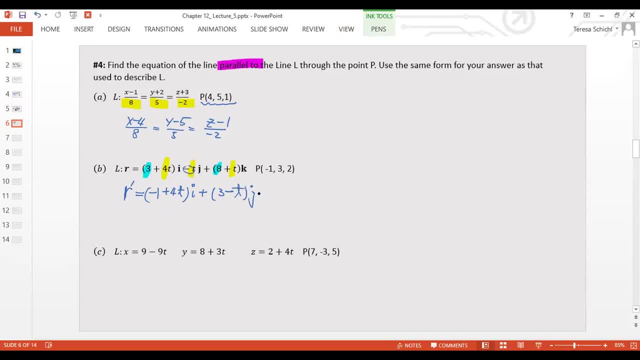 is three, right, so it's three. but i have a is three, right, so it's three. but i have a minus t here, minus t here, minus t here, minus t the j, and what is the third one? minus t the j and what is the third one? 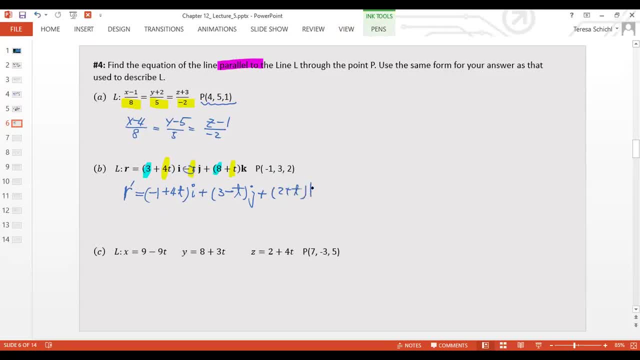 minus t the j. and what is the third one? we replace two, we replace two, we replace two. two plus t with the k. so it's pretty two plus t with the k. so it's pretty two plus t with the k. so it's pretty straightforward, straightforward. 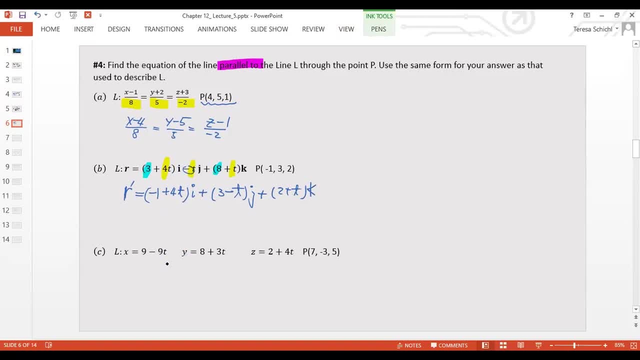 straightforward: all right, all right, so the now. all right. all right, so the now. all right, all right. so the now. number c is here. so what uh? number c is here. so what uh. number c is here, so what uh. so this is. oh, i'm sorry, this is a. 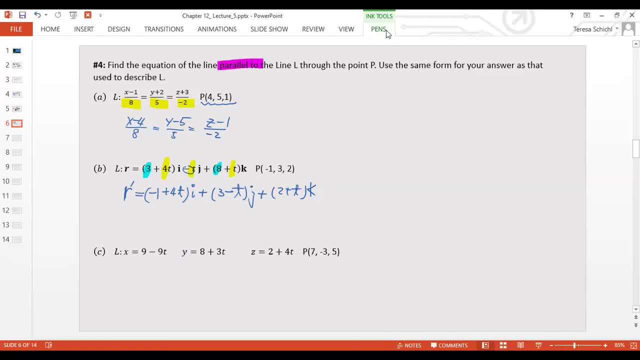 so this is: oh, i'm sorry, this is a. so this is: oh, i'm sorry, this is a symmetric form. this is a parametric form. symmetric form. this is a parametric form. symmetric form. this is a parametric form. so a parametric form. first, let's. 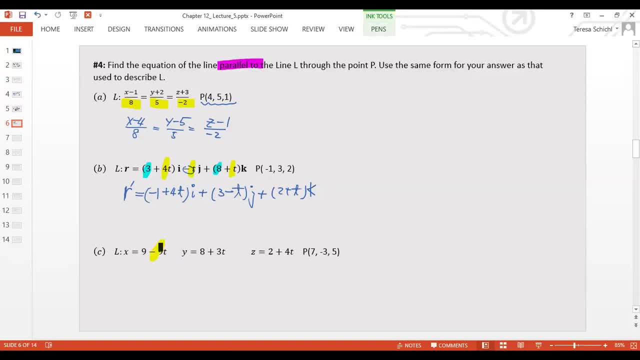 so a parametric form first. let's so a parametric form first. let's recognize the where recognize the. where recognize the? where is my directional vector? here is my directional vector. here is my directional vector, here, here and here. okay, so now this one is here and here. okay, so now this one is. 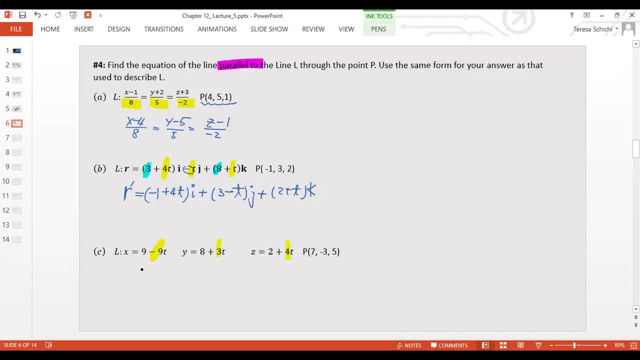 here and here. okay, so now this one is pretty easy, pretty easy, pretty easy to do so. what is the answers here? so to do so? what is the answers here? so to do so? what is the answers here? so x equal to what, x equal to what, x equal to what? 7 minus 90. 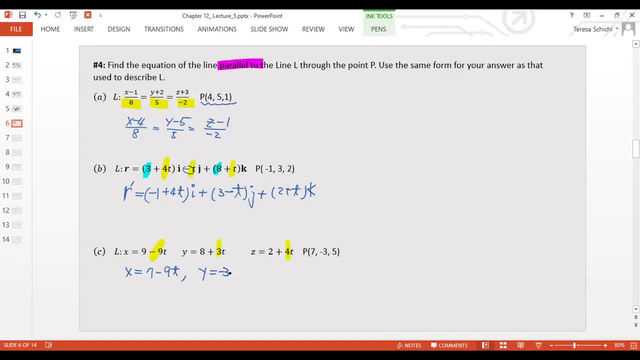 7 minus 90, 7 minus 90 y, equal to what negative 3 plus 3t and the z negative 3 plus 3t and the z negative 3 plus 3t and the z is equal to what two water is equal to what two water. 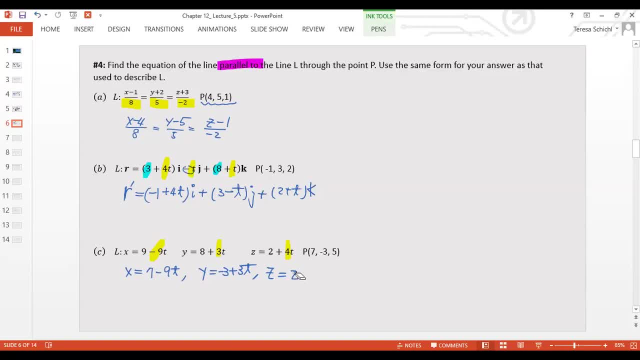 is equal to what two water? i'm sorry, it's not a. two is the new. i'm sorry, it's not a. two is the new. i'm sorry, it's not a. two is the new points right? so it's a. what is a? five points? right, so it's a. what is a five? 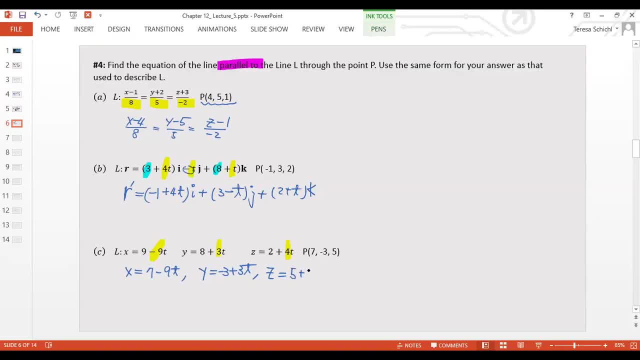 points. right, so it's a. what is a five? it's right, so it's a five. it's right, so it's a five. it's right, so it's a five plus four t. it's right, so they all have. plus four t. it's right, so they all have. 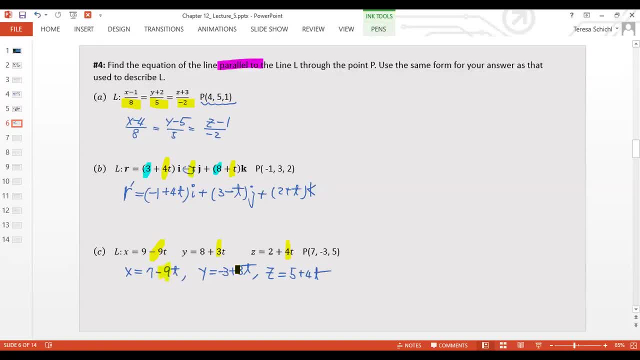 plus four t, it's right, so they all have the same, the same, the same the direction right, so negative. nine, the direction right, so negative, nine. the direction right, so negative. nine. three, three, three and the four. okay, so now the and the four okay, so now the. 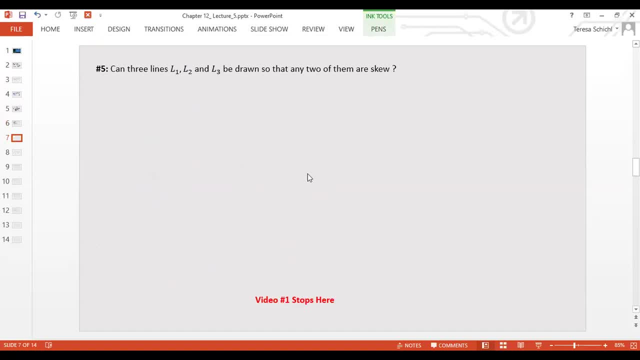 and the four. okay, so now the okay. so here before we finish these. okay, so here before we finish these. okay, so here before we finish these videos, videos, videos here. so the last problem is so they say: here, so the last problem is. so they say: here. so the last problem is so they say: hey, can three. 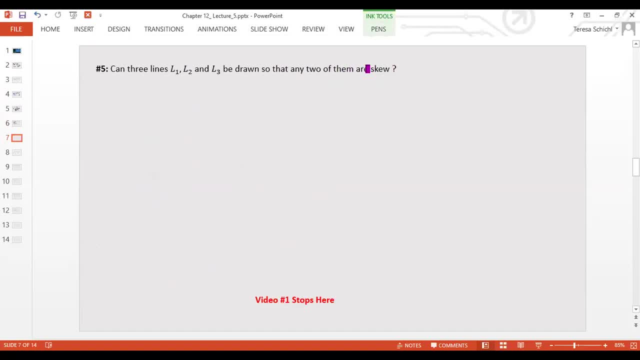 hey can three, hey can three lines right draw. so two of them: lines right draw. so two of them lines right draw. so two of them that any two of them are always the that. any two of them are always the that, any two of them are always the skews. 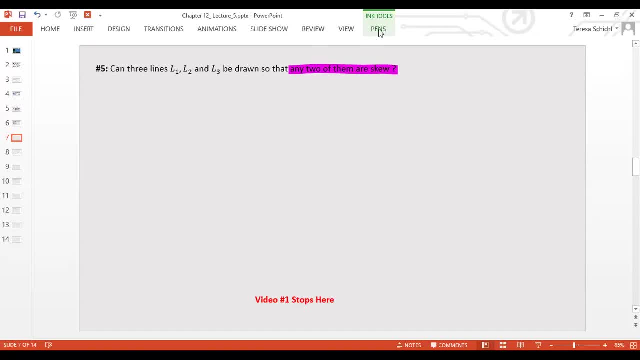 skews, skews here, okay. so in fact, this one here: okay, so in fact, this one here, okay. so in fact, this one is a pretty, is a pretty, is a pretty interesting. the true often is always interesting. the true often is always interesting. the true often is always skew right. so let's take a look here. 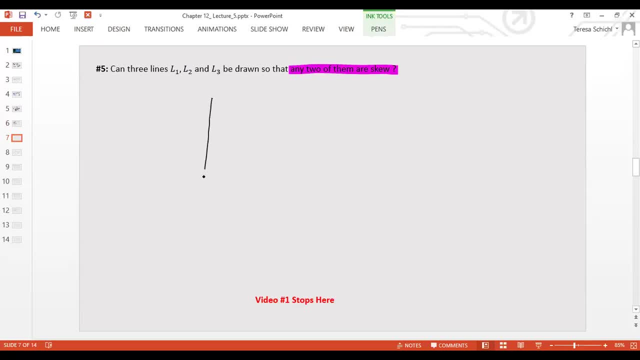 skew, right, so let's take a look here. skew, right, so let's take a look here. okay, so let's see what is the skew. so okay, so let's see what is the skew. so okay, so let's see what is the skew. so here, this is the z-axis. 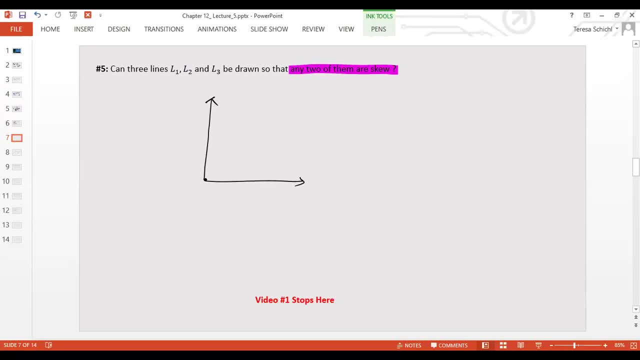 here, this is the z-axis, here, this is the z-axis and this is the y-axis, and this is the y-axis and this is the y-axis. and let's say: here, this is the x-axis. and let's say: here, this is the x-axis. and let's say: here, this is the x-axis. here. 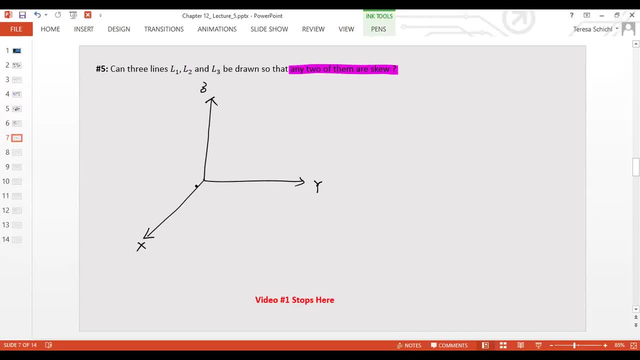 here here. okay, okay, okay, let me try to do a first one here. let me try to do a first one here. let me try to do a first one here. let's see here: this is one, two, three. let's see here: this is one, two, three. let's see here: this is one, two, three, four. one, two, three, four. 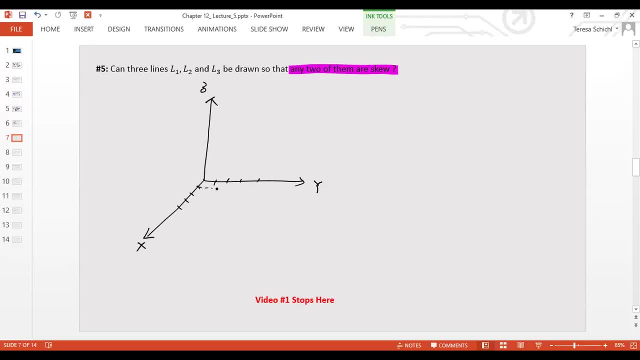 four, one, two, three, four, four, one, two, three, four. that's all right. so let's do the first. that's all right. so let's do the first, that's all right. so let's do the first. one, one. one is one and two here, this one, see here. 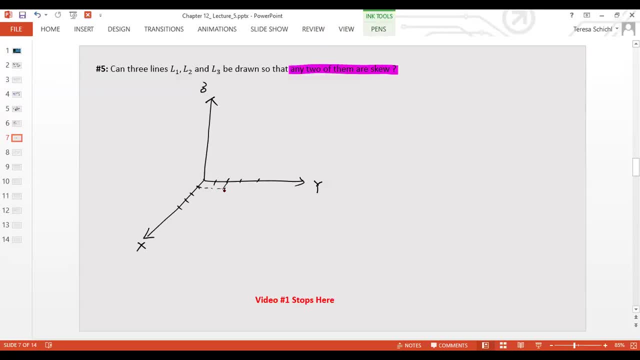 is one and two here. this one, see here, is one and two here. this one, see here. so i'm drawing a line, so i'm drawing a line, so i'm drawing a line. sitting here, sitting here, sitting here, the red one goes through, the red one goes through. 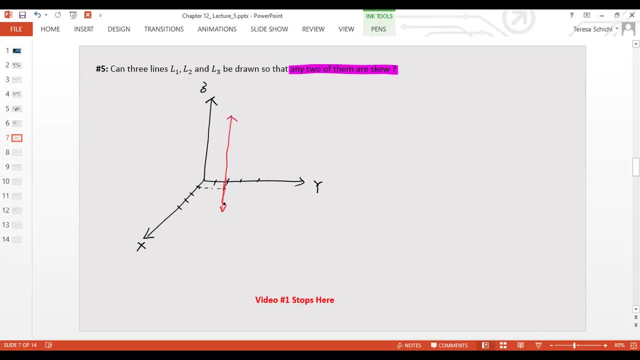 the red one goes through punches through the x y planes and the punches through the x y planes and the punches through the x y planes and the parallel, parallel, parallel to the z axis here, okay, to the z axis here, okay, to the z axis here, okay, so i can do, and other lines, here one 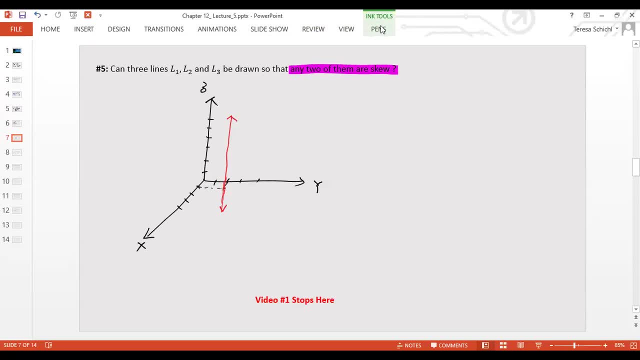 so i can do. and other lines here: one, so i can do. and other lines here: one, two, three, four, five, six. let's try to do two, three, four, five, six. let's try to do two, three, four, five, six. let's try to do another one, another one. 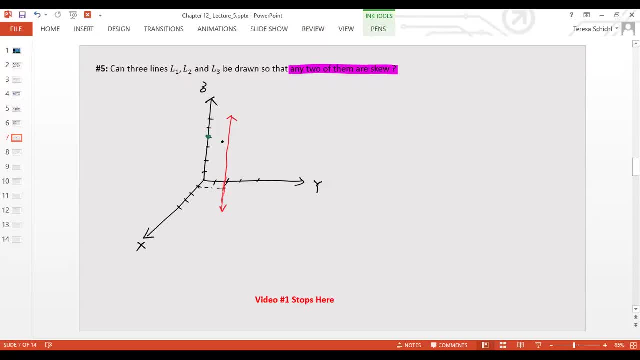 another one. i say one, two, three, four. i do a one. i say one, two, three, four, i do a one. i say one, two, three, four. i do a one. go through the z, go through the z, go through the z right, so go through the z right, so go through the z. 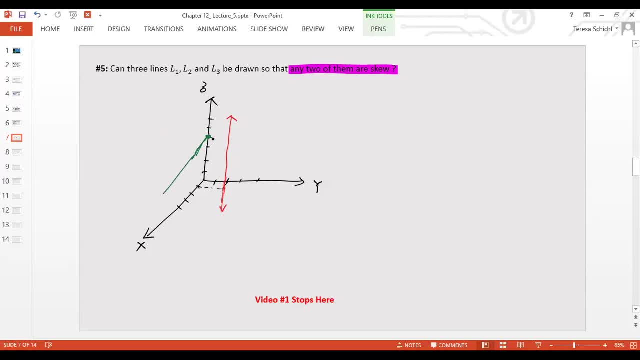 right. so go through the z axis right and axis right and axis right and parallel to parallel, to parallel to the x-axis, the x-axis, the x-axis. okay, so now, okay, so now, okay. so now i can, i can, i can do the other ones here, do the other ones here. 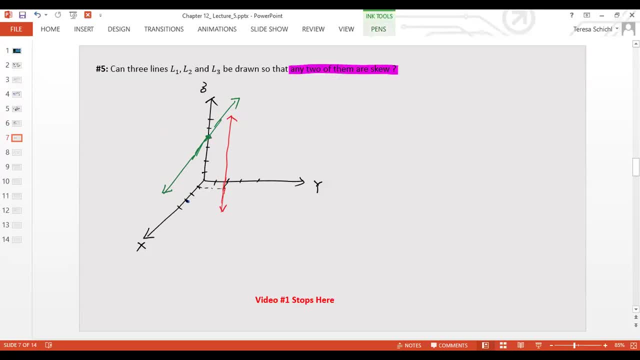 do the other ones here. okay. so i say here, this is the threes. okay. so i say, here, this is the threes. okay. so i say here, this is the threes, right, so this is the three here. right, so this is the three here. right, so this is the three here. now i go to. 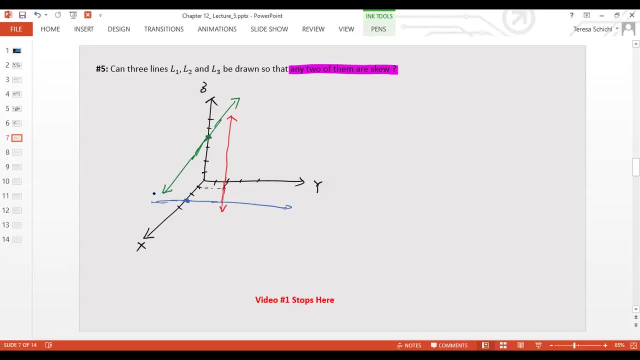 now i go to, now i go to do a line here, do a line here, do a line here, right, so can you right, so can you right, so can you visualize that, visualize that, visualize that. so any two of these lines, they are skewed. so any two of these lines, they are skewed. 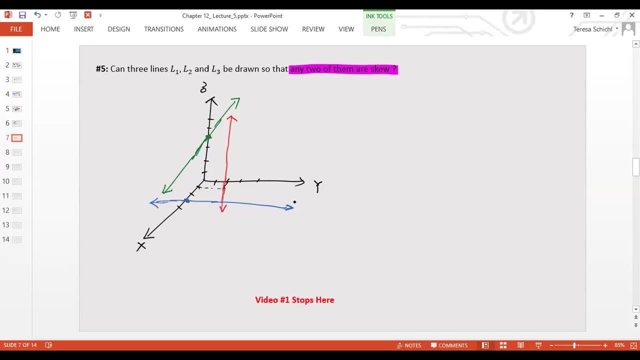 so any two of these lines, they are skewed. so for example the red one. so for example the red one. so for example, the red one and the blue one say here: right. so the and the blue one say here: right. so the and the blue one say here: right. so the red one and the blue one, they are not. 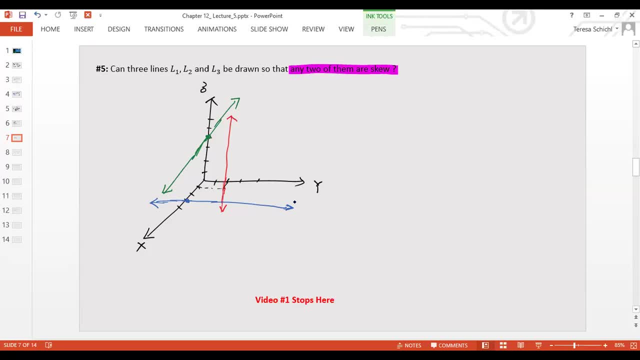 red one and the blue one. they are not red one and the blue one, they are not parallel, but they're not going to touch parallel. but they're not going to touch parallel, but they're not going to touch in my graph it's kind of like little. 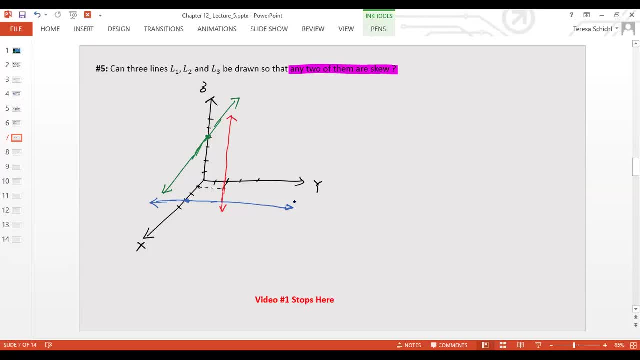 in my graph it's kind of like little. in my graph it's kind of like little touch but it's not touch, but it's not touch, but it's not right because they're going to go through right, because they're going to go through right, because they're going to go through the xy plane at the. 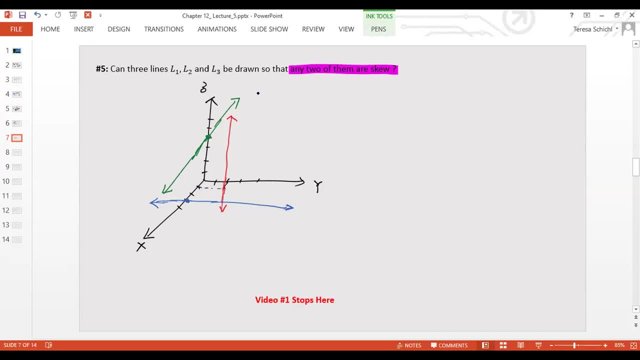 the xy plane at the, the xy plane at the, when the x equal to ones here. so when the x equal to ones here, so when the x equal to ones here. so basically, if you want to, so this is basically if you want to, so this is basically if you want to. so this is not really go like this, right? so this? 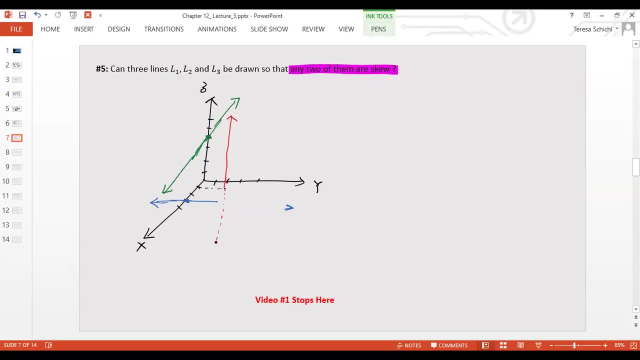 not really go like this, right. so this not really go like this, right. so this one's here, one's here, one's here it's kind of like. then this part is it's kind of like, then this part is it's kind of like: then this part is going down right, so it's going. 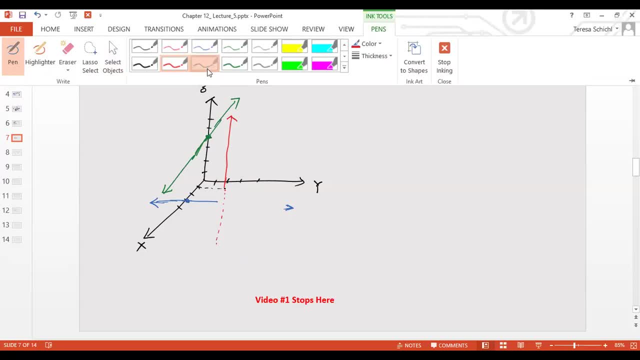 going down right, so it's going going down right, so it's going piece. you know kind of the go through piece. you know kind of the go through piece. you know kind of the go through. you know the go through the xy planes. you know the go through the xy planes. 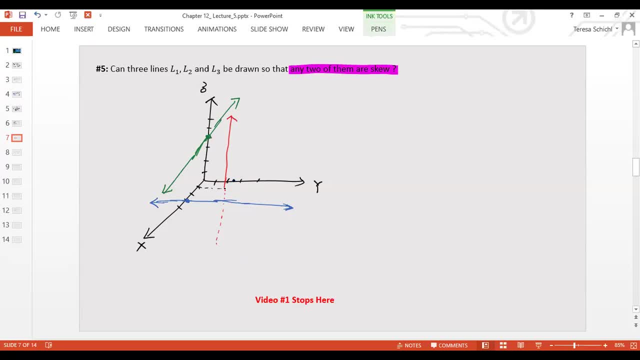 you know, the go through the xy planes. here that's one, the blue one and the red. here that's one, the blue one and the red. here that's one, the blue one and the red one is not going to, one is not going to, one is not going to touch here, right? so the same way is. 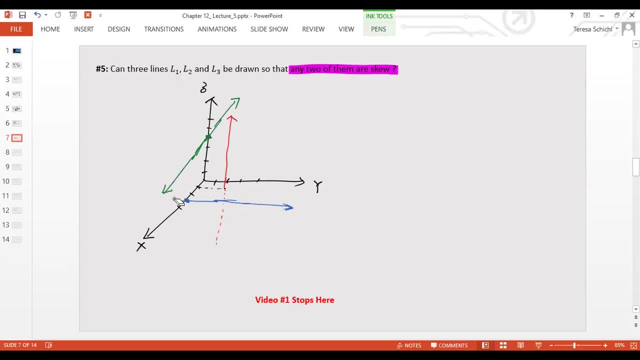 touch here, right. so the same way is touch here, right. so the same way is here for the blue ones here, here for the blue ones here, here for the blue ones here. this one's here, really, you know it's. this one's here, really, you know it's. 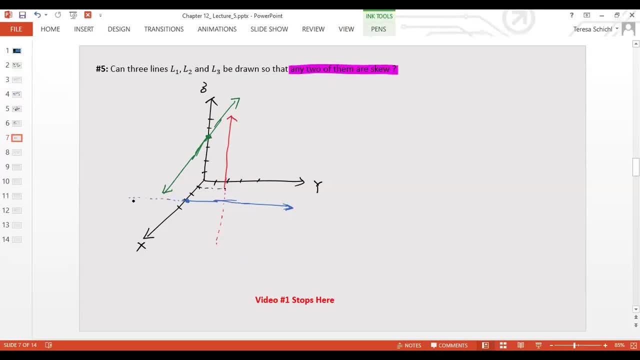 this one's here. really, you know it's going through like this one. you see the going through like this one. you see the going through like this one. you see the bottom line. see here, bottom line, see here, bottom line, see here. that's why they kind of pass, you know. 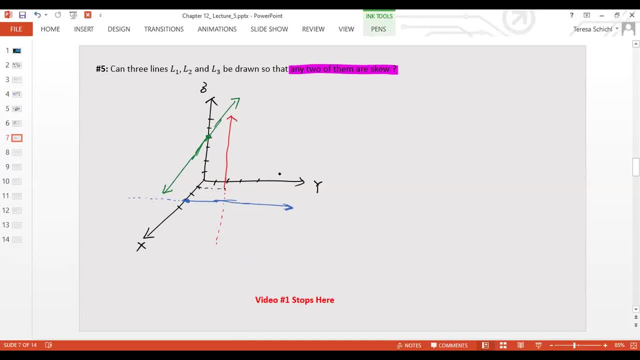 that's why they kind of pass, you know, that's why they kind of pass, you know, kind of parallel to the y, but in here kind of parallel to the y, but in here kind of parallel to the y, but in here this is, this is, this is. so the blue one and the green one, they 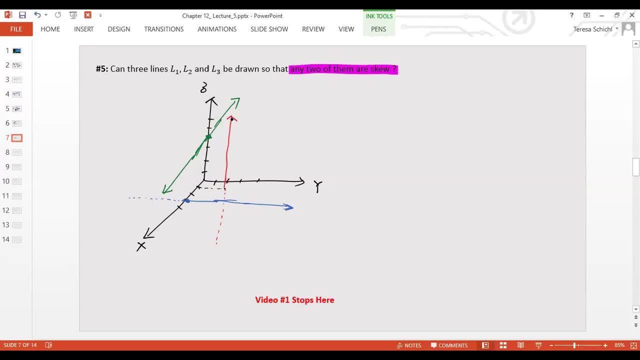 so the blue one and the green one. they so the blue one and the green one. they are apparently so. this type of the lines are apparently so. this type of the lines are apparently so. this type of the lines we called, we called, we called, are the skew right, so the any two of. 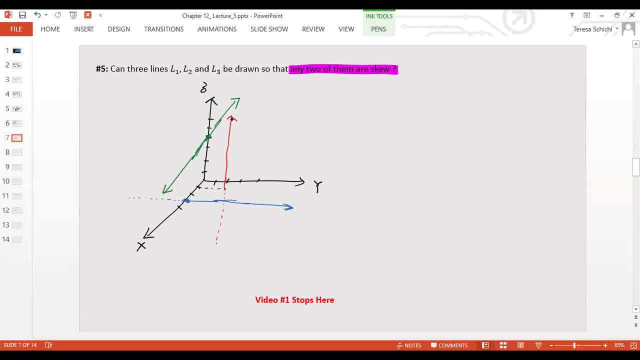 are the skew right. so the any two of are the skew right. so the any two of them, they are skewed to each other. them, they are skewed to each other. them, they are skewed to each other. okay, that's it so like uh right now. okay, that's it so like uh, right now. 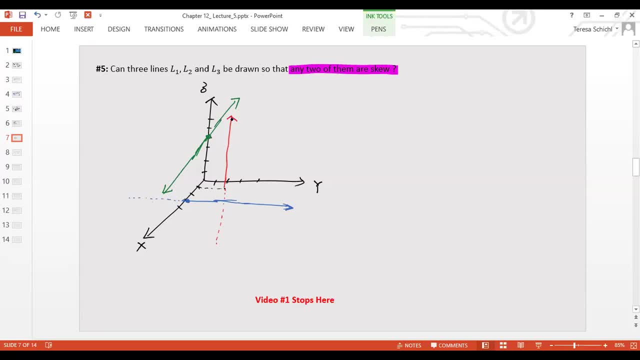 okay, that's it. so like, uh, right now we're going to stop, we're going to stop, we're going to stop here. so we know how to write a line here. so we know how to write a line here. so we know how to write a line in the r3s, right, so the in the r3. 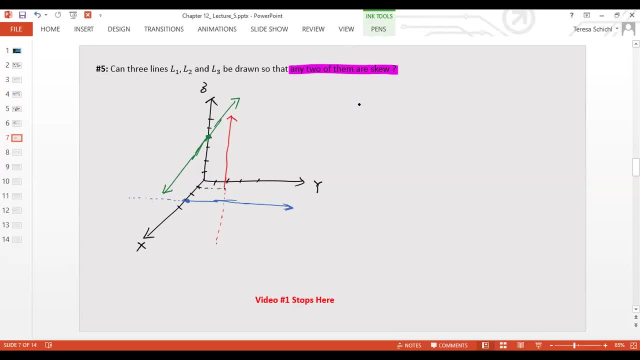 in the r3s, right, so the in the r3 you know. so that refreshes what we you know. so that refreshes what we you know. so that refreshes what we learn. we have three forms: the vector learn. we have three forms. the vector learn. we have three forms: the vector form, parametric form. 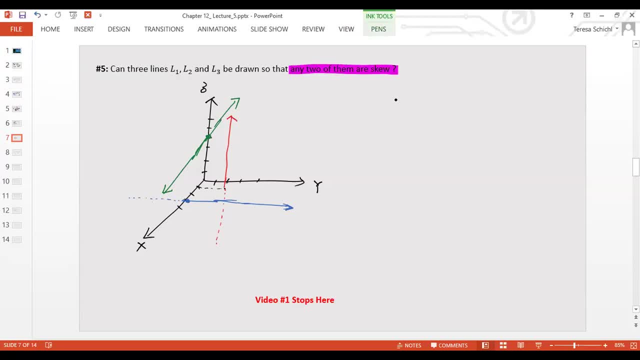 form, parametric form, form, parametric form and what. and symmetric form and what and symmetric form and what and symmetric form, also in the r3. you know if you remember also in the r3, you know if you remember also in the r3, you know if you remember in r2.